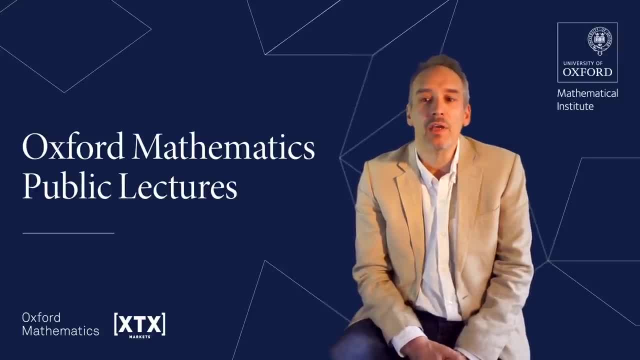 models. This evening I'm very happy that Robin Thompson has agreed to talk to us about his issues. Robin is currently a junior research fellow in mathematical epidemiology at Christchurch College and a member of the Mathematical Institute. Robin has been modeling infectious diseases. 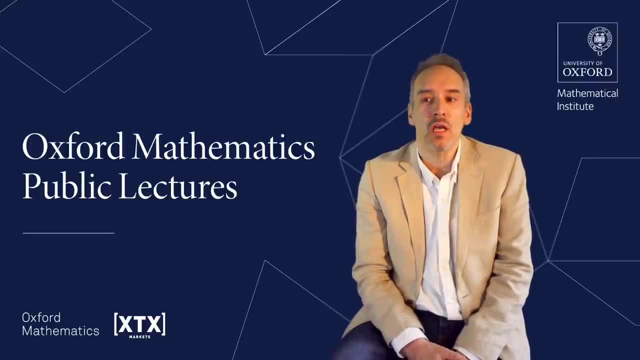 for several years and since early January he has been working on important questions about coronavirus forecasting and control. Since then, he has been extremely busy contributing to the national modeling effort and making appearances in media about topics including social distancing and COVID-19 outbreak risk. If you would like to ask questions, 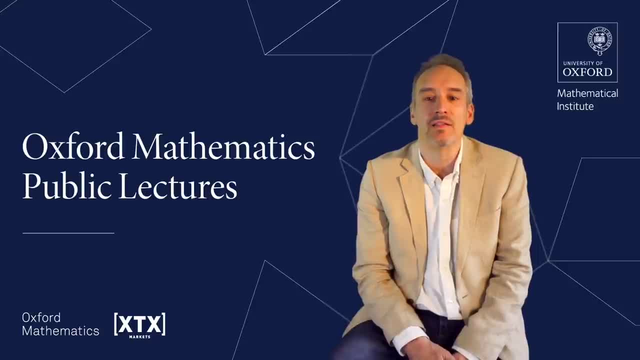 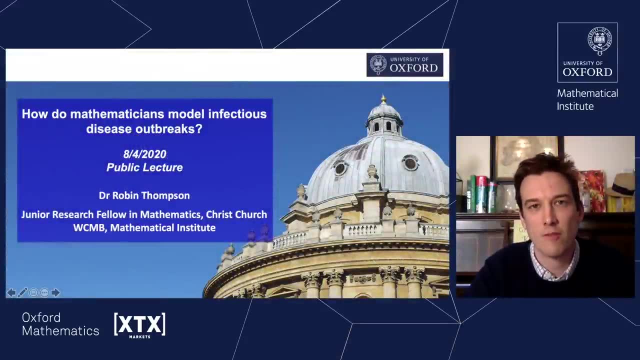 send it in via social media and we will collate them and send out answers in the next couple of days. Thank you, Robin, Thanks Alain And hello everybody. Welcome to this Mathematical Institute public lecture, which is coming live from my home here in Oxford. My name is Robin Thompson. I'm a 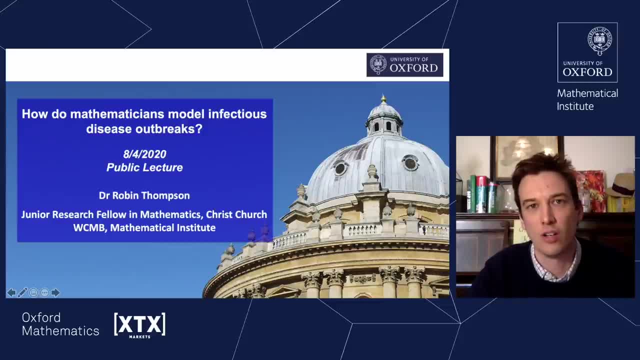 junior research fellow at Christchurch and I also work in the Mathematical Institute in the Wolfson Center for Mathematical Biology. My specialist research area is infectious disease outbreak modeling And that's a topic, of course, that's been in news a lot recently, because mathematical models are 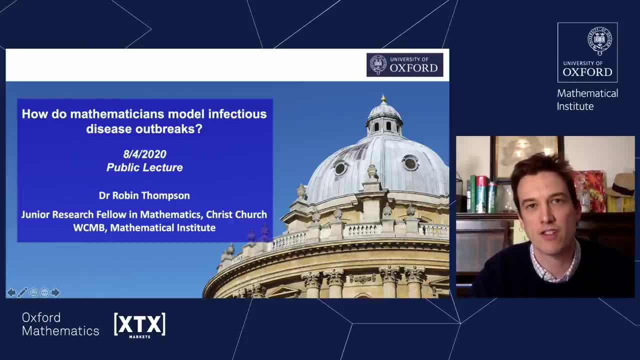 being used in real time to inform public health measures against the COVID-19 outbreak. So what I'm going to do now is I'm going to talk to you about precisely how mathematicians go about modeling infectious disease outbreaks. So the natural place to start, then, is: well, what exactly? 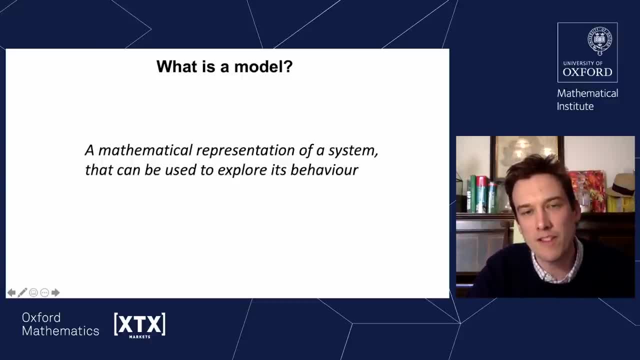 is a mathematical model. Well, a mathematical model is a mathematical representation of a system that can be used to explain the effects of a disease, And it can be used to explain the effects of an outbreak, And then it's an EVP that allows us to explore that system's behavior And the goal. 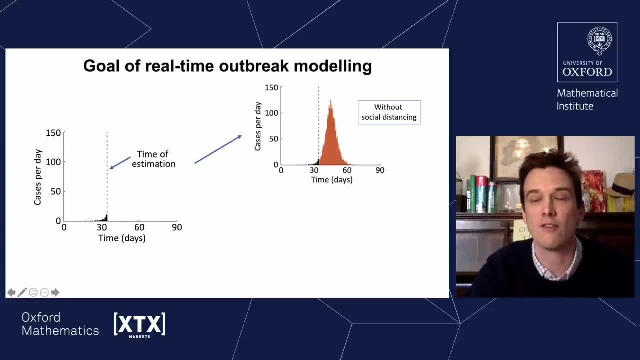 of real-time infectious disease outbreak modeling is as follows. What we do is we look at data from an outbreak so far, So, for example, we might have data on the numbers of cases per day during the outbreak. Then what we do is we construct a mathematical model. 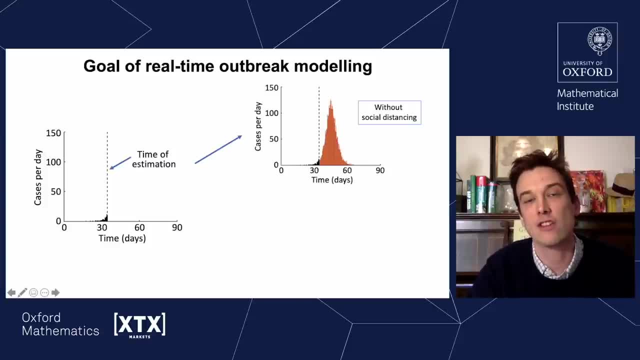 that represents the underlying epidemiology of the system. We then use simulations of the model forwards to predict what might be likely to happen in the future, how many cases we might be expected to see per day going forwards. What we can then do, when we've got a model that can make a sensible forecast, is we can then 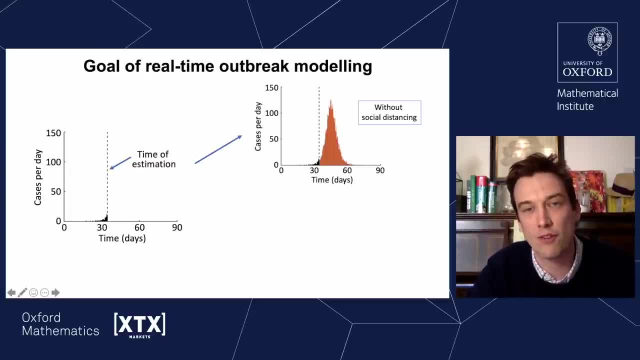 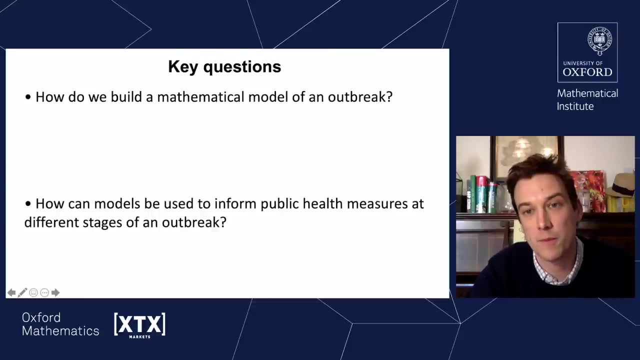 introduce control interventions into the model to look at how different control interventions might affect the numbers of cases that we might be likely to see in future. So during this lecture I'm going to focus on two main questions. The first one is: how exactly do we build a mathematical model of an infectious 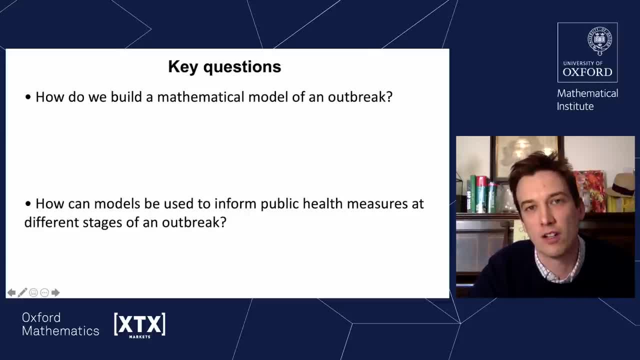 disease outbreak. And then the second question I'm going to answer is: well, once we've got a mathematical model, how can we use it to inform public health measures at different stages of an outbreak? And so these are the kind of sub questions that I'm going to address. The first thing I'm going to address is: 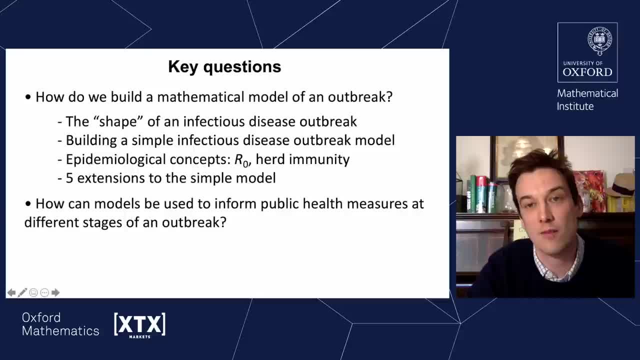 well, is there a characteristic shape of an infectious disease outbreak? and if so, that's something that's interesting because mathematicians are very interested in shapes. Then I'm going to talk about how we can build a very, very basic infectious disease outbreak model. I'll then talk about some epidemiological concepts that 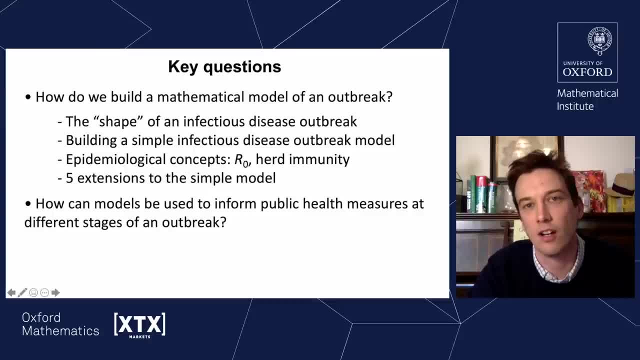 you might have heard about during the COVID-19 outbreak. so far, For example, policymakers have been talking a lot about the basic reproduction number, or R-naught, and the concept of herd immunity has been in the news a lot. so I'll talk about those two ideas. I'll then talk about five ways that the very 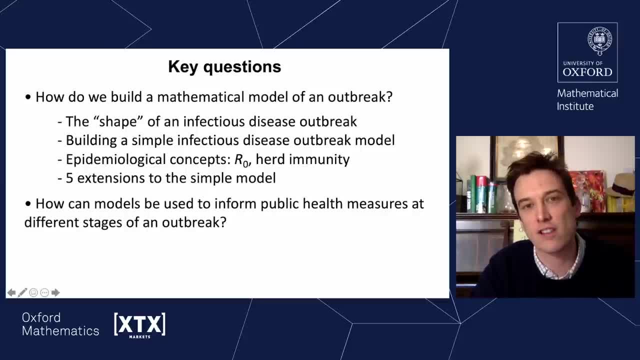 basic infectious disease outbreak model that we're going to use to build a construct can be extended to make them more realistic. And then, after that, I'm going to talk about how mathematical models can be used to inform public health measures. Well, I'm also going to talk about three different stages of an 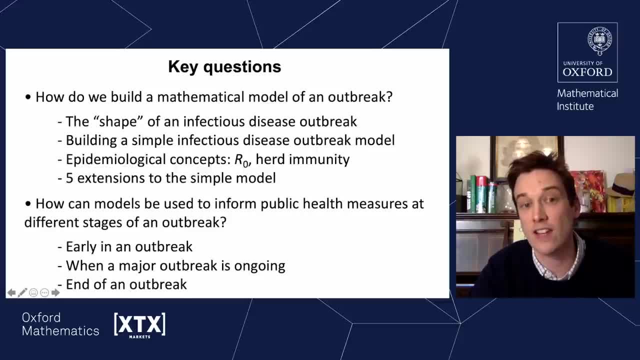 outbreak. So can mathematical models be used usefully early in an outbreak to inform public health measures? Can mathematical models be used when a major outbreak is ongoing? So, for example, in the scenario that we're in at the moment here in the UK and elsewhere around the world? And then, finally, I'll 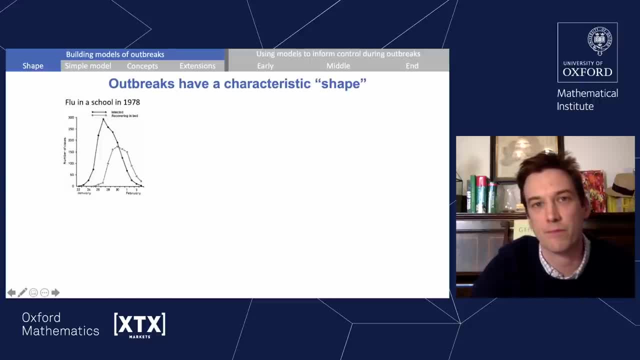 talk about how mathematical models can be used usefully at the end of an outbreak. So the first thing I want to point out is that most single wave infectious disease outbreaks tend to have a characteristic shape, And so here's one example. So this, what you can see here, is a data set of an outbreak of 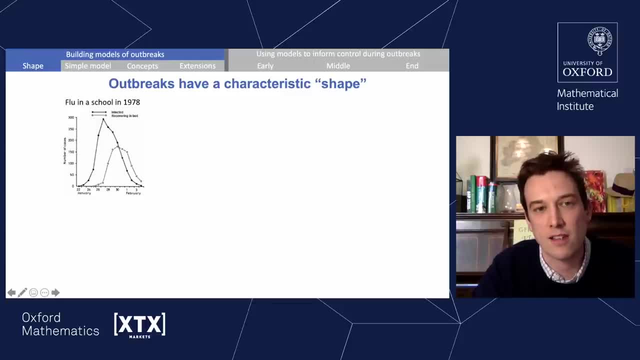 influenza in a boys boarding school in the north of England in the 70s And what you can see is that the virus enters the school, the numbers of cases gradually increase and it increases until there's quite a large number of cases. But it 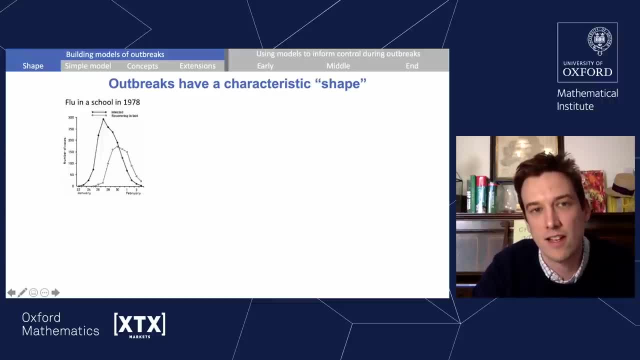 doesn't keep going until everyone in the school is infected. Instead, it slows down again and the outbreak peaks, and then the numbers of cases comes back down again to near zero, And this kind of shape is characteristic of lots and lots of single wave outbreaks. So here's another example. This is the foot and. 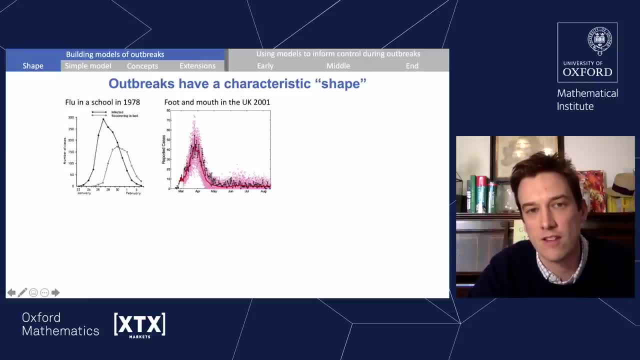 mouth disease outbreak in the UK in 2001.. The data here is slightly different, so it's not individual cases of disease But rather it's the number of infected farms. But broadly you see the same kind of shape. The virus enters the population, it takes off, it goes up to a kind of 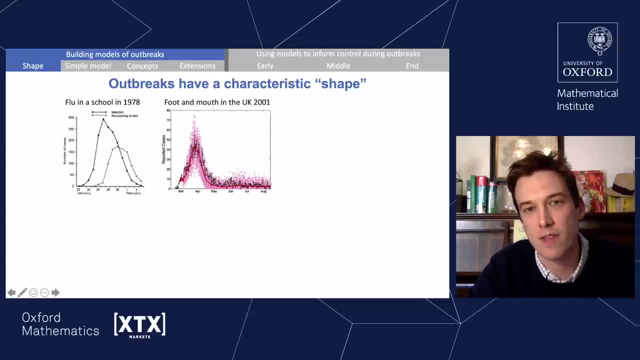 high level in which there are lots of farms that are infected, But then it peaks and comes back down again, back down to near zero. So again, broadly you can see the same kind of shape of an outbreak. The graphs have the same kind of rough shape. The same thing happens if we look at a third example. So this third, 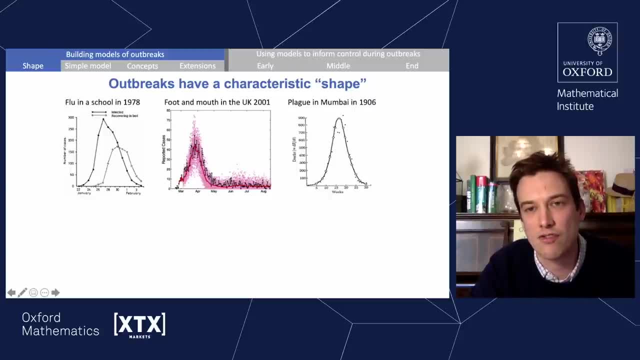 example is plague in Mumbai at the beginning of the 20th century. Again, this is very slightly different data. This is data on the numbers of individuals that were dying during that plague outbreak. But again you see a very similar dynamic in which the number of deaths increases, but it increases up some. 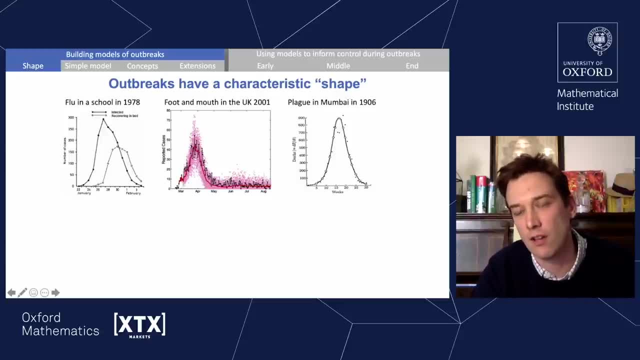 high level, and when it reaches that high level it turns over and falls back down again to near zero. So again, broadly the same shape. Here's a more recent example. This is Ebola in West Africa, the largest Ebola outbreak in history. And again, 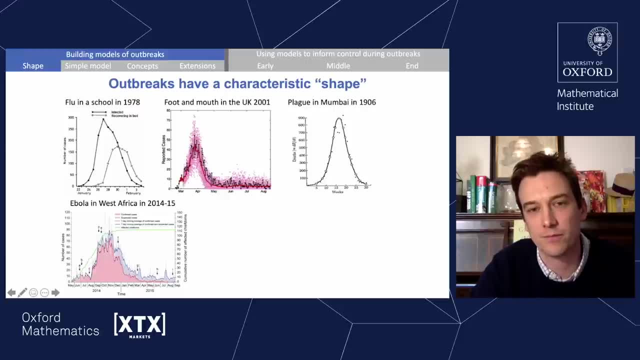 we see a very similar looking outbreak shape And here's one example from the ongoing COVID-19 outbreak. This is data from China, specifically data on the numbers of individuals currently infected in China each day throughout the outbreak, And what you can see again is that the number of cases gradually 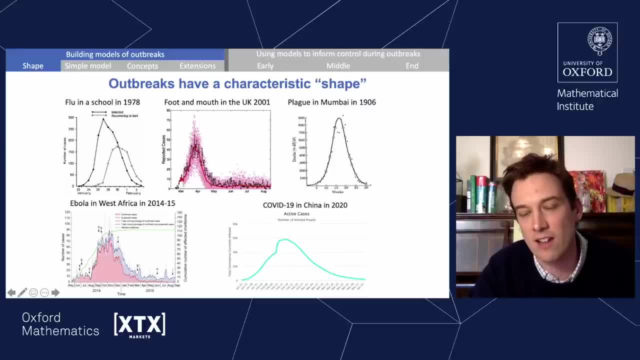 increased. It increased up to some high level again, then it turned over and then the outbreak began to fade out. One particularly interesting feature of that specific graph is that you can see just here, so if you look in mid-February, there's a sudden increase within a 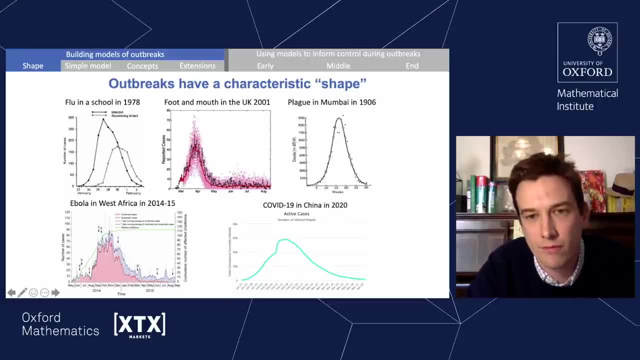 single day in the number of infected people, And the reason for that sudden increase was that precisely what constituted an infected case changed. The definition of a case changed in China during the COVID-19 outbreak. So before that time, in order to be counted in the data, you actually had to be tested. 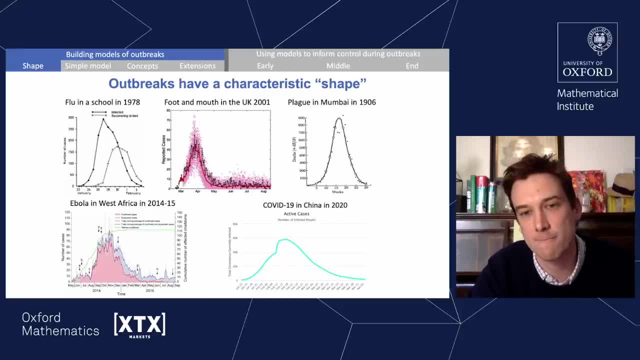 and found to be carrying the novel coronavirus. But obviously when case numbers are very high, it's very difficult to go and test everybody. And so what happened then was there was an assumption that, because case numbers were high, if you develop symptoms that were consistent with infection by the 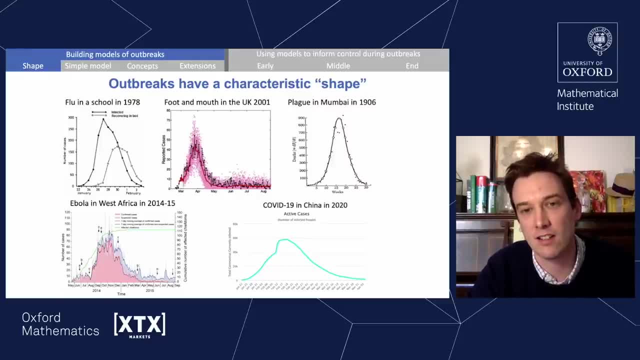 novel coronavirus. then you were included in the data And so suddenly, because of this change in definition, you no longer had to be actively tested and found to be carrying the virus. The numbers of cases shot up very suddenly, But despite that, broadly you can see the same kind of shape In this case, the 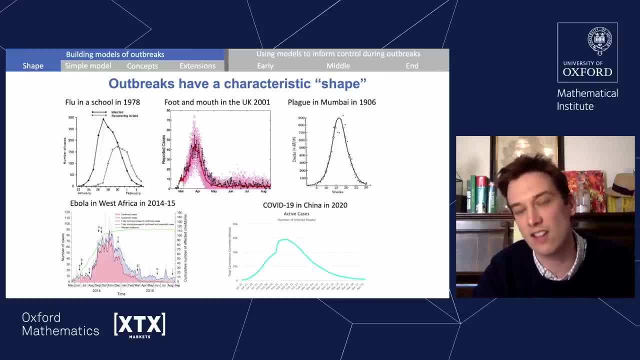 virus invades, it goes up some high level, then the numbers of cases turns over and falls back down again to near zero. And you can see that, no matter what kind of outbreak data you're looking at in these graphs, whether you're looking at deaths, 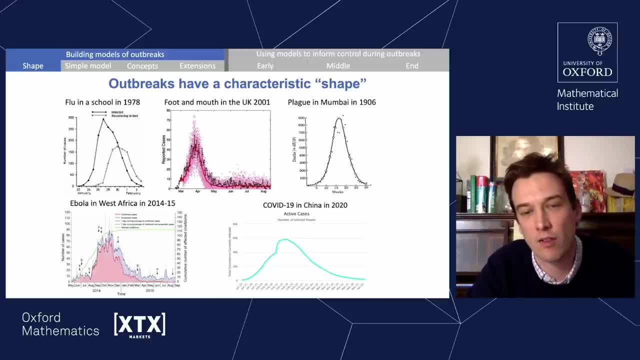 or number of infected farms, as in the case of foot and mouth, or number of individual cases, like in the flu example, or like in the COVID-19 example. So outbreaks have a characteristic shape and what we want to do is we want to recreate that shape. 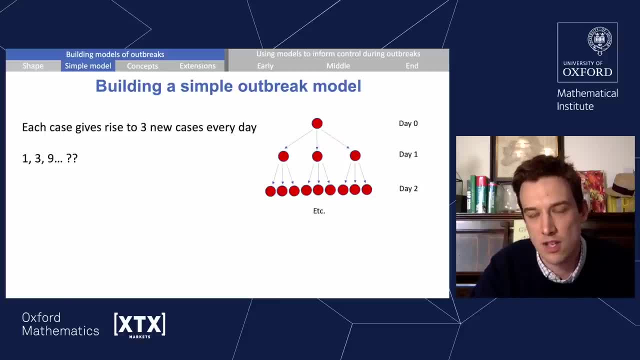 using a mathematical model. So what we could do if we wanted to is we could make the simplest possible assumption about how an infectious disease spreads. The simplest possible assumption would be to assume that every single case of disease leads on to some fixed number of new cases every day. let's say This is 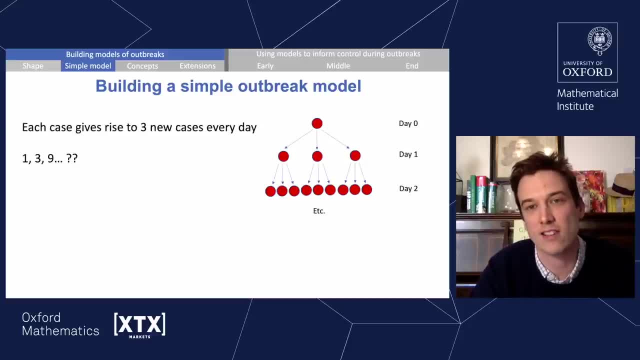 one example. so we're going to assume that each case gives rise to three new cases every day. Well then, at the beginning of the outbreak, so in day zero, you might just have one infected individual. On day one, that one infected individual will have. 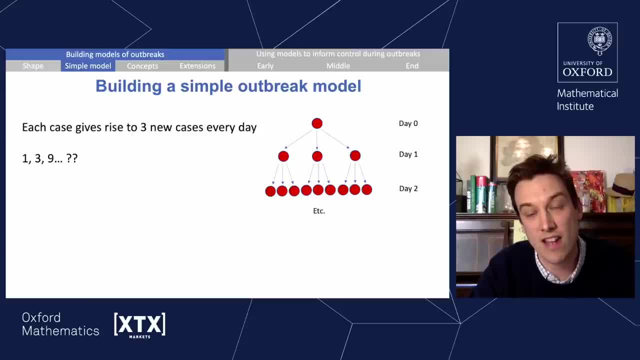 gone and infected three other individuals. So on day one need have three new cases. Then, according to this very basic model, we assume that on day two each of the three cases from day one will have generated three new infections each. So in other words, on day two you've got nine new cases and then 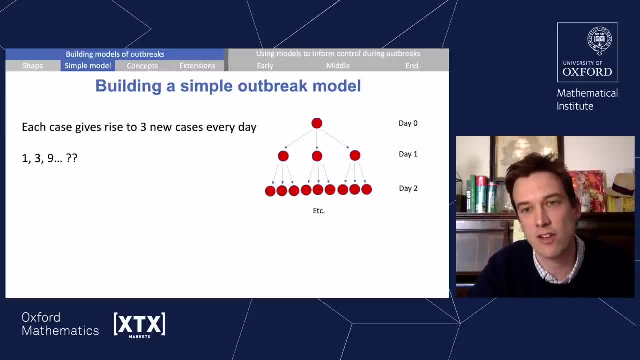 on day 3. each of nine would cause three new infections. so you'd have 27 new infections on day three, and so on and so on. You can imagine this would just carry on going. And so the assumption of this model. so this model is called a geometric progression. 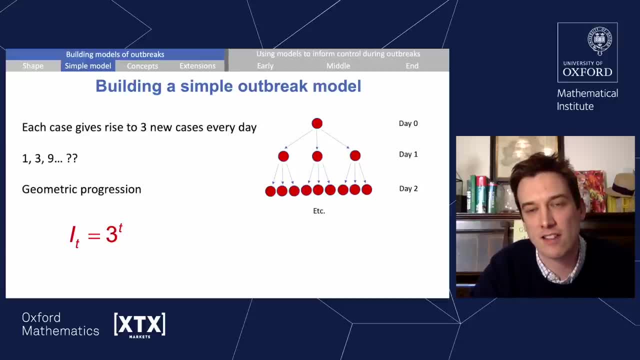 what you'd find if you looked for a formula describing the numbers of cases on day t is you'd see that the formula was just equal to three to the power of t. that's the number of new cases on day t. So when t equals zero, the number of cases is three to the power of zero. 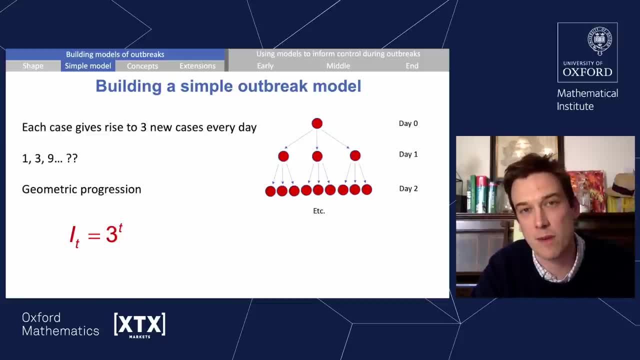 which is one. On day one, the number of new cases is three to the power of one, which is three. On day two, the number of new cases is three to the power of two, which is nine, and so on. So this is the simplest possible infectious disease outbreak model. 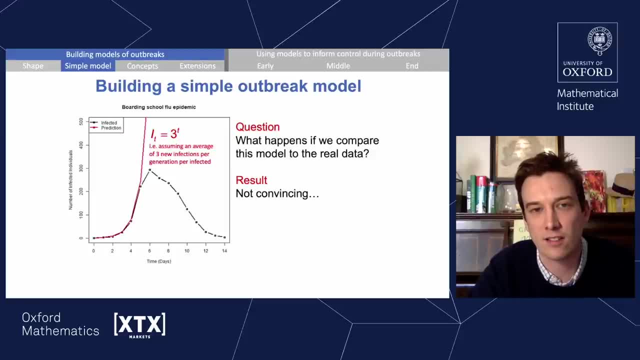 Well, does this actually look anything like real world data? So what I've done here on this graph is I've plotted the data from the boys boarding school flu epidemic that I showed you a moment ago, and the data are plotted in black. So the 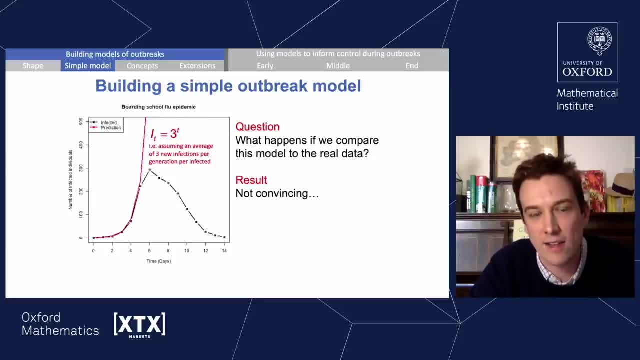 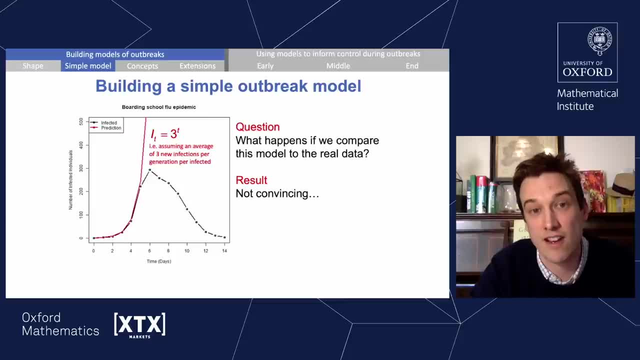 individual infects three new individuals every day, And if we overlay that, what we can see is that actually the model does a pretty good job of representing the very early parts of the infectious disease outbreak. The red is matching the black very well early on in the outbreak, But 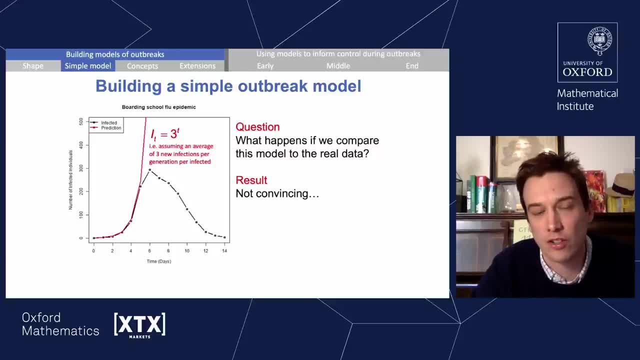 later on in the outbreak, then the mathematical model isn't doing a good job at all. The numbers of cases in the model is shooting off up to infinity, Whereas if you look at the infectious disease outbreak data, the data, like we just saw, turns over and comes back down again to near zero. 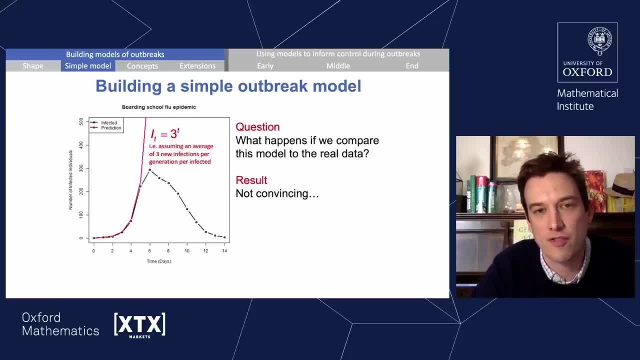 So the model prediction isn't doing a particularly good job of capturing the data. So what we have to do next, then, is a very important aspect of mathematical modelling. What we have to do next is we have to refine the data. So what we have to do next is we have to refine the data. So what we 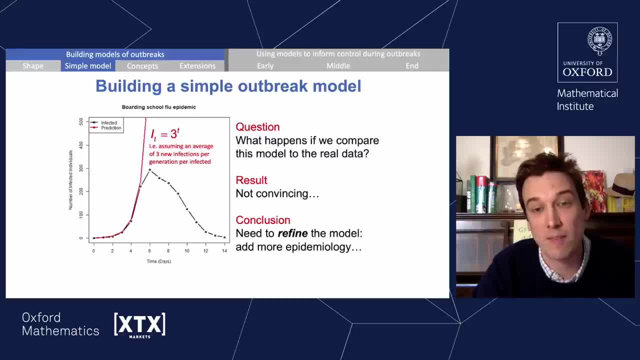 have to do next is we have to refine the data. So what we have to do next is we have to refine the model. We can't just carry on with this model. We have to make it better, make sure that the model matches the data more closely. We have to add in more infectious disease epidemiology. 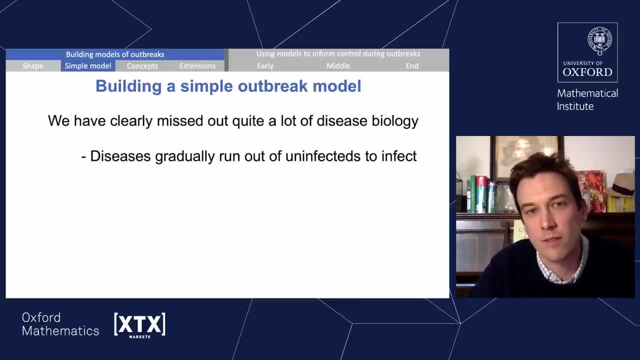 So clearly, one of the issues with this very basic model is that we've missed out a huge amount of disease biology And, in particular, we've missed out the fact that diseases gradually run out of uninfected susceptible individuals to infect, And so what we can do instead is we 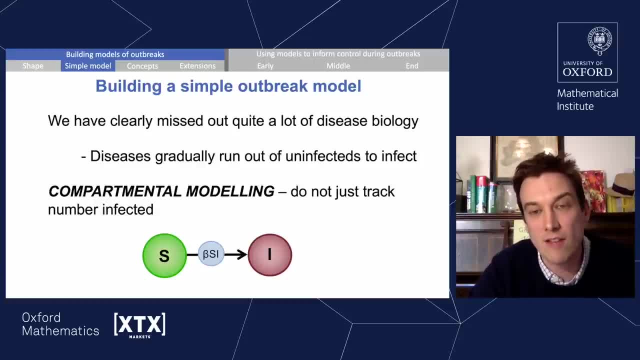 can consider what's called compartmental modelling, And the idea of compartmental modelling is that you don't just keep track of how many individuals are infected, You keep track of individuals with all different infection and symptom statuses. So the simplest possible compartmental model- 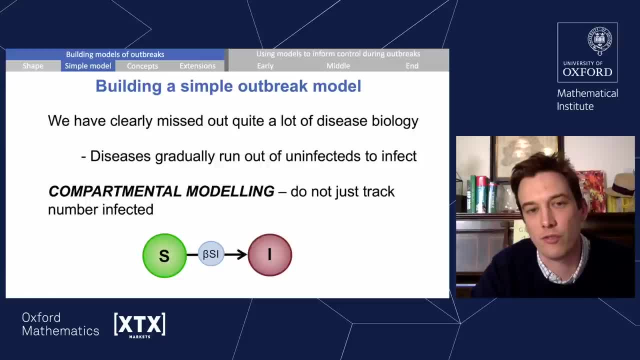 you can develop is this model here. This is called the SI model, And so in the SI model, what you do is you divide individuals according to whether they're susceptible to the disease, in which case they're in the S compartment, they're in the green. 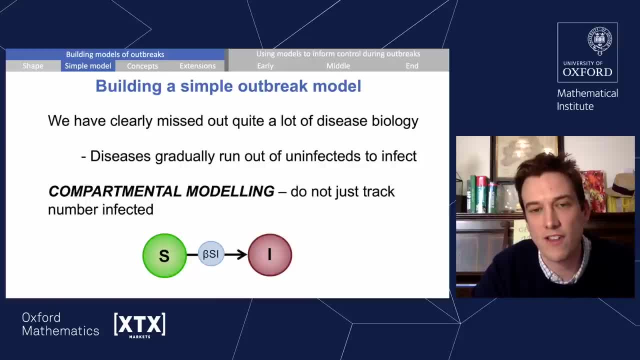 circle on the left, Or an individual can be infected and generating new infections. And if an individual is infected, then they're in the red circle, they're in the eye compartment, they're in the red circle on the right And as you simulate an infectious disease outbreak using this model, 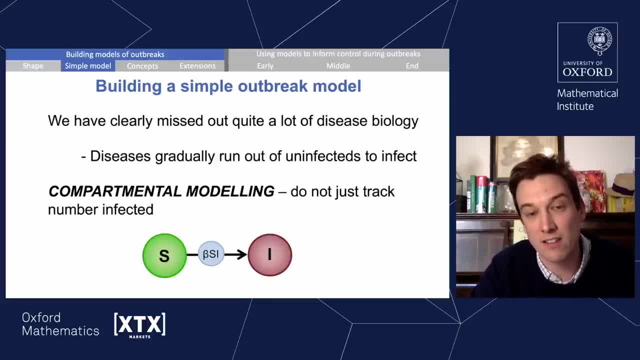 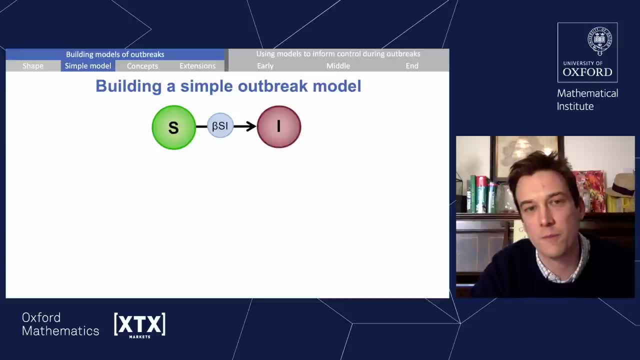 what you would see is you'd see individuals that are susceptible becoming infected. So, in other words, you'd see susceptible individuals from the green circle transitioning over into the red circle. So this is the SI model that I just described. We can write down equations for this particular. 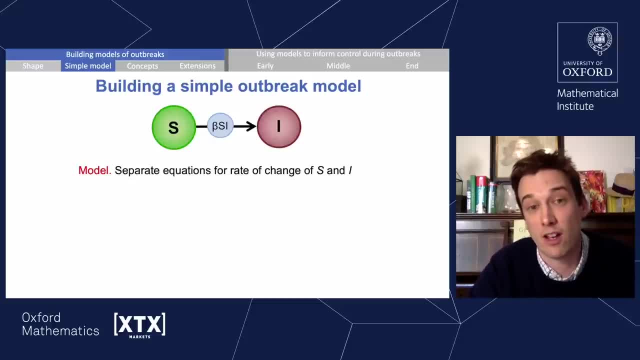 model, And so it doesn't really matter if you know whether the key point of this is the idea of compartmental modelling. It's not the precise equations, But for those of you that are interested in the equations, I'm going to show them. So what we have is we have two separate equations. One: 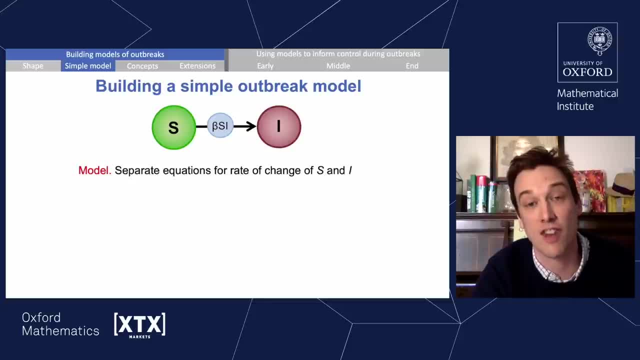 equation describes the rate of change of the number of susceptible individuals And the other equation describes the rate of change of the number of patients, Of the number of infected individuals. So we write down two equations that look a little bit like this. So, like I say, it doesn't matter if you haven't met equations like this before On the 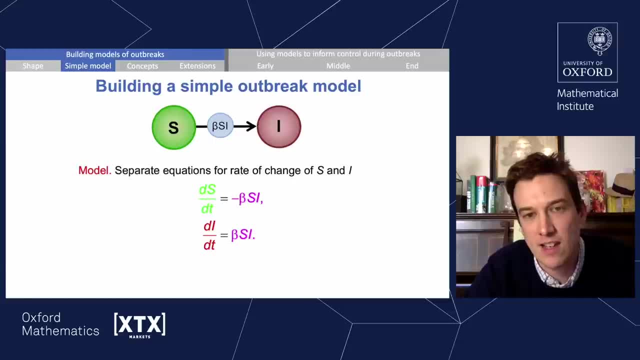 left hand side. this term here, this ds by dt, that just means the rate of change of the number of susceptible individuals, And this term here is something that's negative. That's why we've got a minus sign just here on the right of the equation And the reason that the rate of change 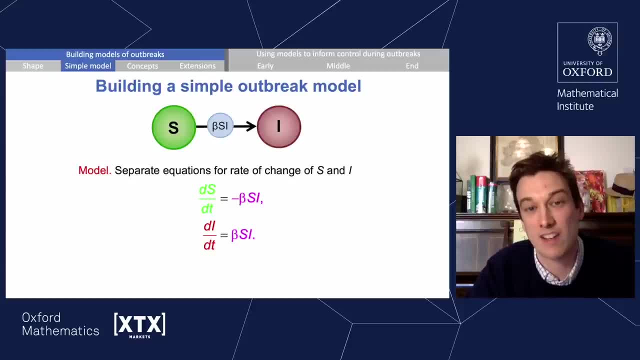 of the number of susceptible individuals is negative is because the number of susceptible individuals decreases during the outbreak as susceptible hosts become infected. Similarly, what we have at the bottom is we have an equation here for the rate of change of the number of infected individuals, And the number of infected individuals is something that 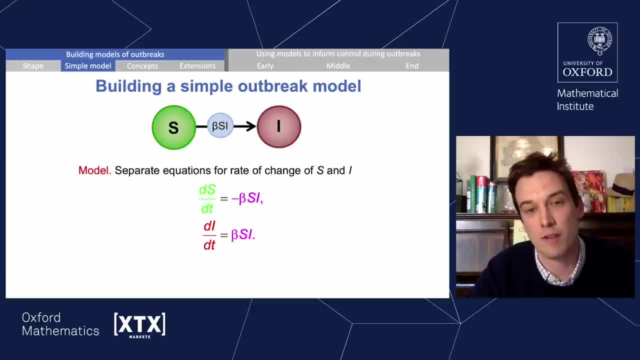 increases during the outbreak as infections happen, And so the rate of change of the number of infected individuals is something that's positive. That's why they're negative. There's no negative sign on the right hand side of this equation, And, in particular, then the overall rate of infection is given by this. 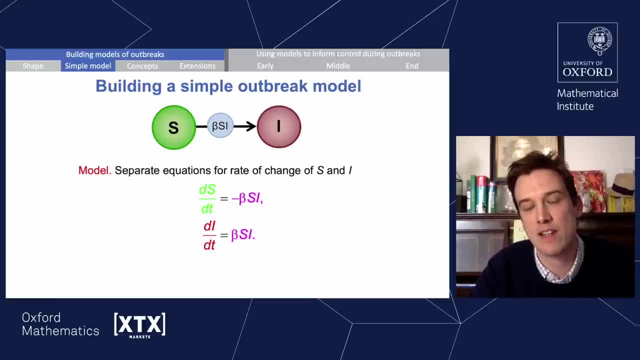 beta si. This is the rate at which the number of susceptible individuals decreases and the rate at which the number of infected individuals increases, And that rate is proportional to both s and i. So the infection rate is proportional both to how many susceptible individuals we've got, but also how many infected individuals we've got. 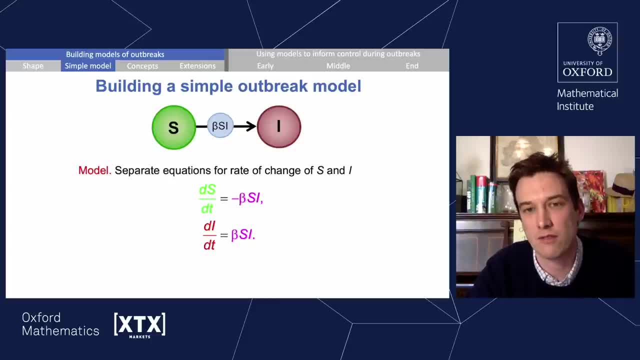 And the reason for that is that if there's a large number of susceptible individuals, then there are lots of people that are targets for the disease. There are lots of people that the disease could infect, And so we'd expect the infection rate to be high. Similarly, if there are lots of infectious, 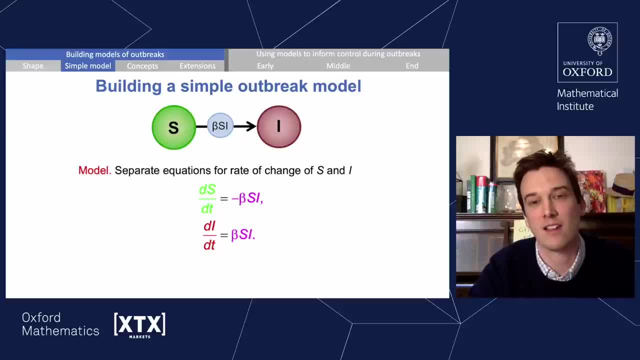 individuals, then there are lots of individuals that can do the infecting, And so, again, if there are lots of infectious individuals, we'd expect the overall infection rate to be high. Okay, so this is the model. So, like I said, ds by dt, the green term is: 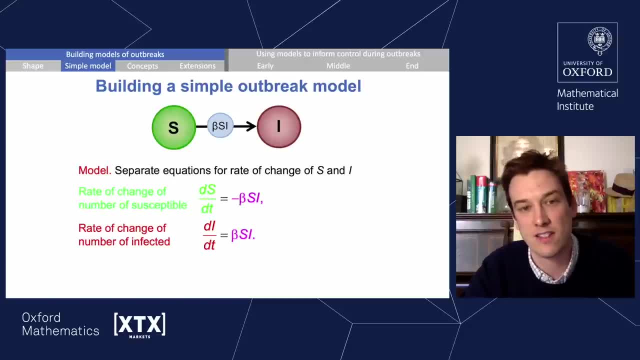 just the rate of change of the number of susceptible individuals. Di by dt is the rate of change of the number of infected individuals, And then we have an overall rate of new infections which is given by beta times s, times i, And that depends on exactly how. 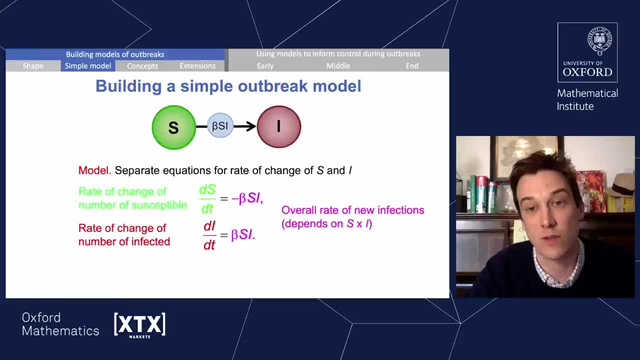 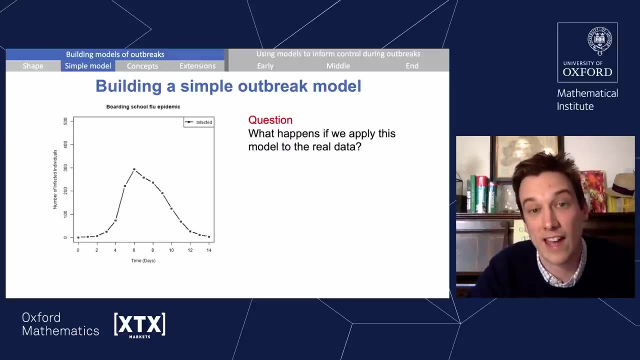 many susceptible individuals we've got and how many infected individuals we've got. And the parameter beta governs the rate of infection, That governs the rate at which individuals become infected. Okay, so what happens Then if we apply this very basic outbreak model again to the real data? 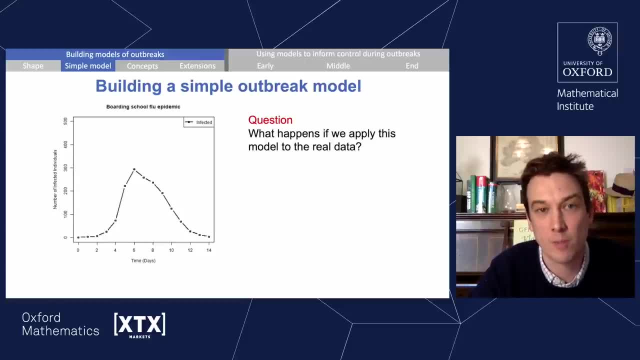 Well, in black. what we have here is we have the data from the boys boarding school flu epidemic in the 70s And what we can do is we can plot the results of this SI model on top of the data. So what you see here is that it does a better job than before. So the red line matches the 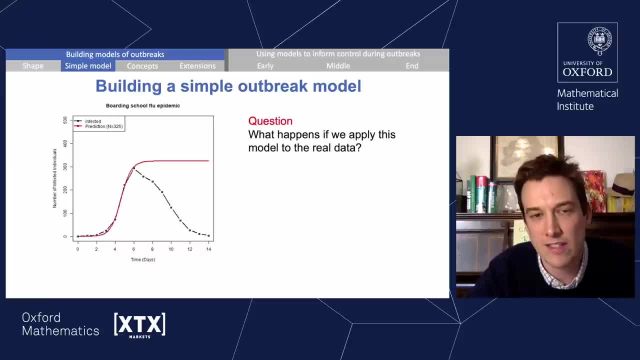 data. So the red line is the model prediction that matches the data pretty closely, But it only does ability to go for about half the outbreak. What happens, like we saw earlier on, is that the data comes back down again. the number of cases declines back down to near zero, Whereas the 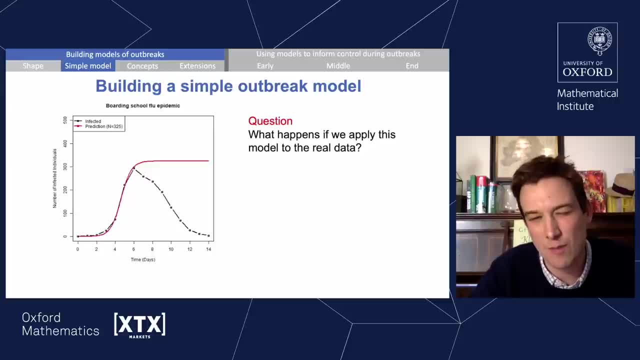 model output, the red line just stays flat, So it doesn't capture the decline in the number of cases. So what we found is that the epidemic- according to our model, the red line- no longer grows without bound. It doesn't go off to infinity anymore, so that's a good thing. 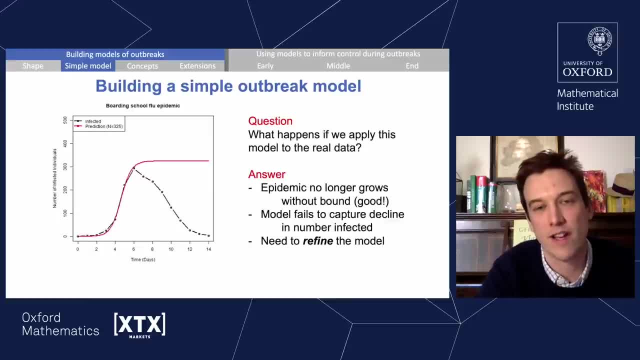 But, like I said, the model doesn't capture the decline in the number of infected hosts. So again, we need to do what we did before, which is we need to refine the model further to try and get the model to match the outbreak data even better. 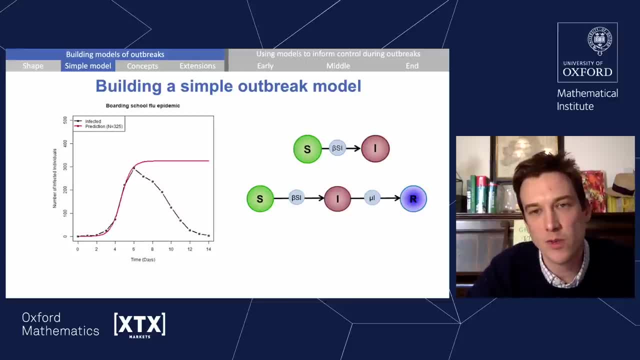 So what we're going to do is we're going to include even more disease biology here. So before we were looking at the SI model, which just accounted for susceptible individuals and infected individuals. what we're going to do now is we're going to include another. 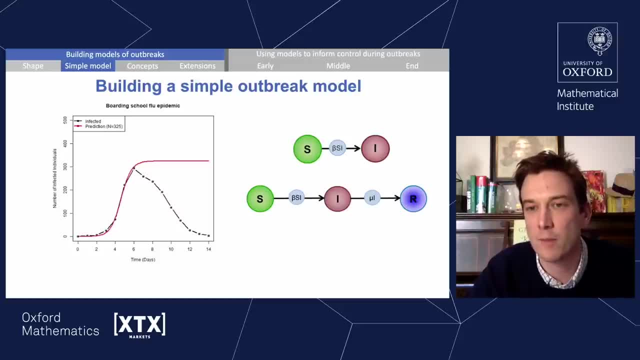 type of individual and they're individuals that have recovered and become immune to the disease and they're in this R class that you can see in the bottom model there. So you have susceptible individuals. when they get infected, they become infected individuals. 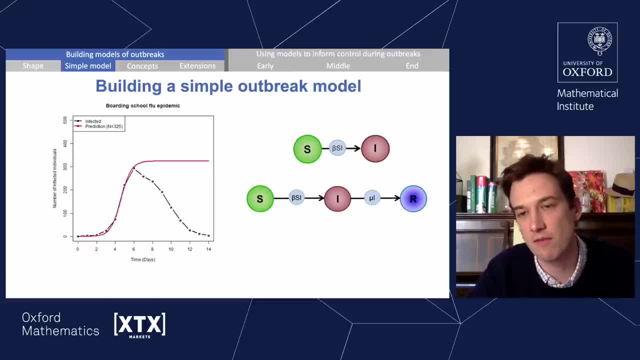 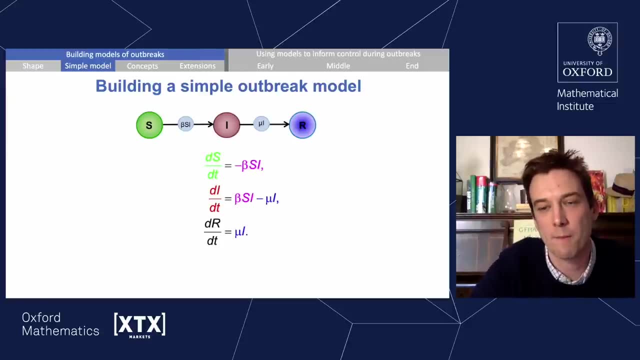 and when they recover. when the infected individual recovers, they become a recovered individual and in this R class And this new model is called the SIR model. OK, so here's the model. We can again write down a set of equations describing the rate at which individuals pass. 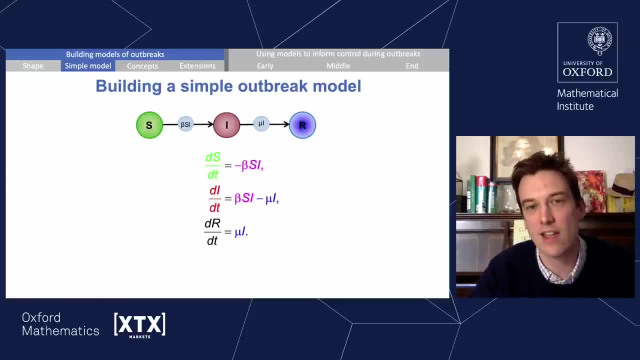 from one compartment into another. So this is exactly the same as the SI model, but we have one new feature, and that new feature is that we have this term here, this mui term, and that mui term is the rate at which infectious individuals recover and become immune to the disease. 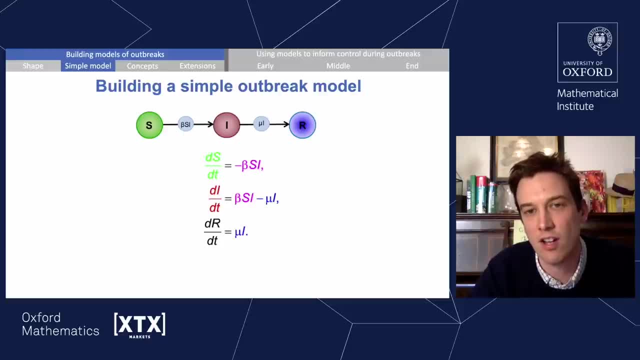 And that term is only proportional to the number of infected individuals there are, And the reason for that is that if there is a large number of infected individuals, then we'd expect to see a large number of recoveries in the near future. OK, 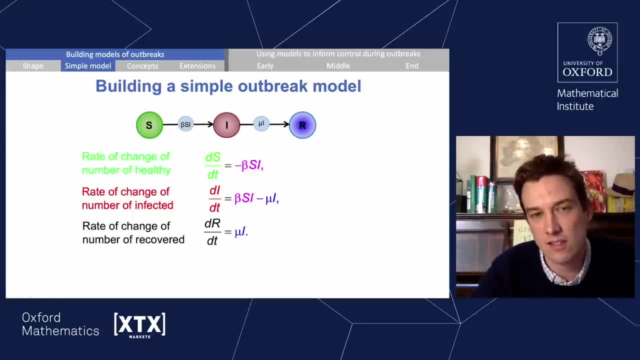 So this is the SIR model. So again, we've got three equations this time. This time it's for the rate of change of the number of healthy susceptible individuals, rate of change of the number of infected individuals and then rate of change of the number of recovered. 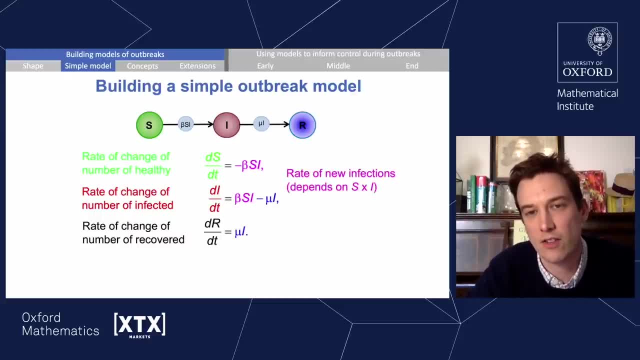 individuals. We can write down the rate of new infections, which is the pink term that depends on S and I, and we can write down the rate at which infected individuals recover and become immune. That's this mui, And so now we've got two parameters. 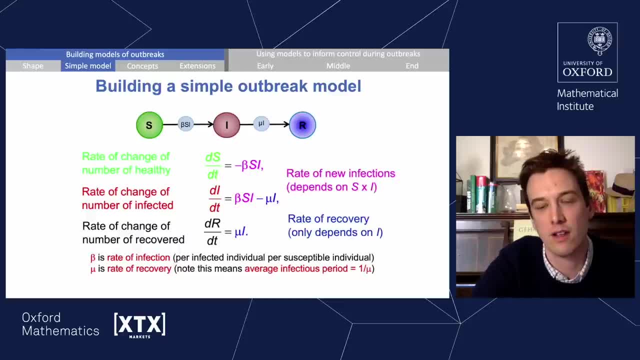 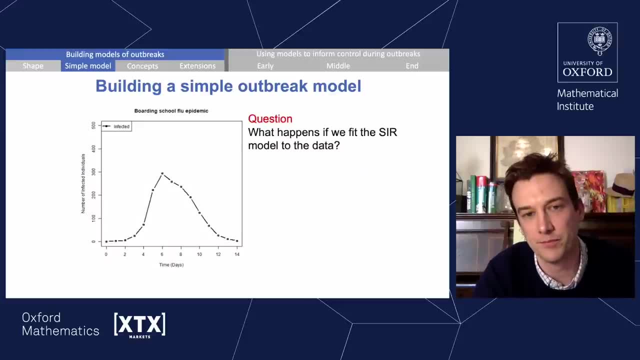 We've got beta, which governs the rate of infection, and we have a new parameter, mui, which governs the rate of recovery, so the rate at which infectious individuals recover. So what happens now, then, if we fit this model to the data? 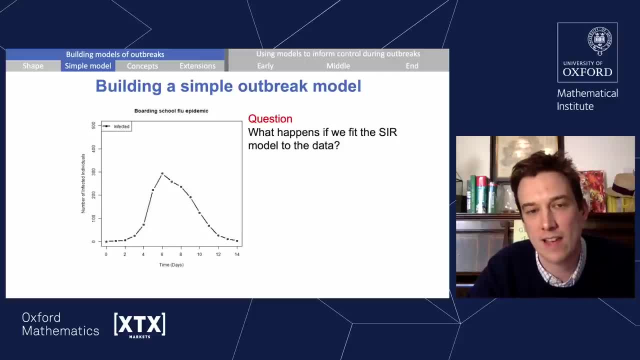 So again, here we have the boys boarding school flu epidemic data set in black and we can plot the results of this new model, and what we see in red is the results of this new model. OK, So what we see is that the red line, the model output, matches the infectious disease. 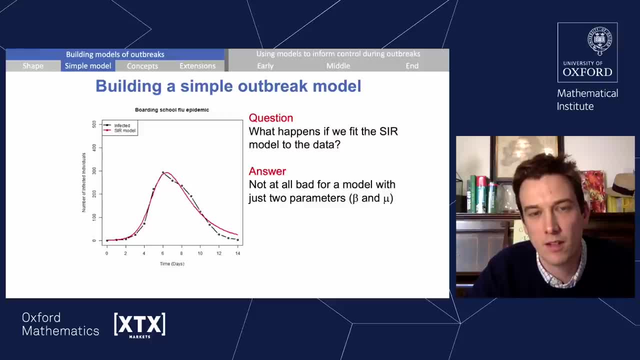 outbreak data pretty closely and I think you'll agree that this actually the model's doing a pretty incredible job, given how simple it was. It was pretty simple to construct that model and the model only included two parameters. There was a parameter governing the infection rate, which was beta, and there was a parameter 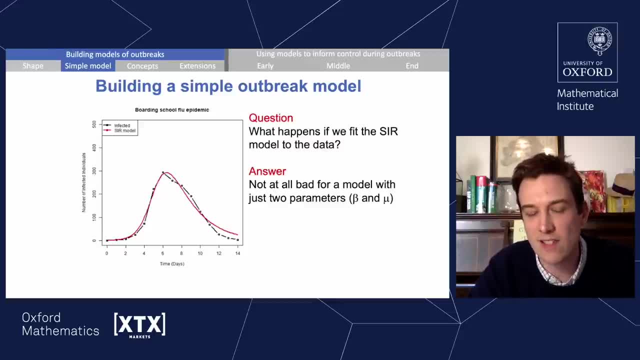 governing the recovery rate, which was mui, but it was a very simple outbreak model and the model output matches the data very well. So the important conclusion is that by refining this model- so we started with one model, we refined it twice and eventually we included recoveries and that allowed us to capture. 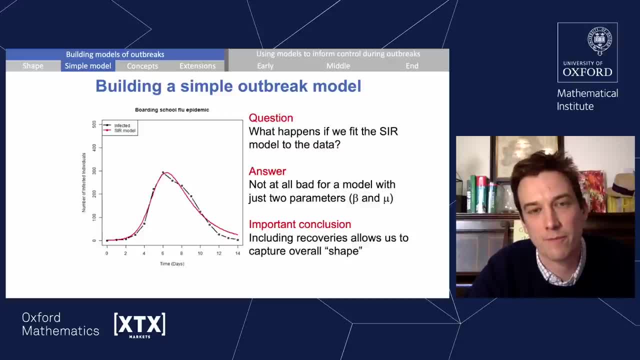 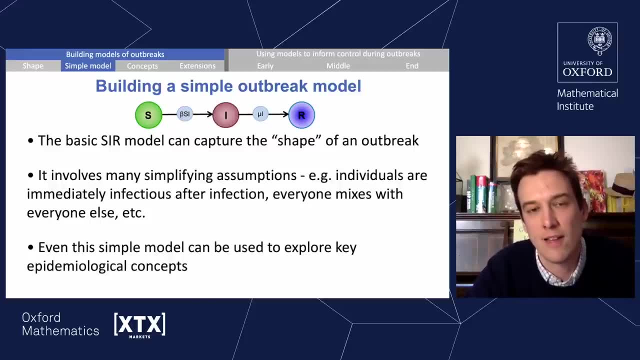 the overall shape of an infectious disease outbreak. This basic SIR model is kind of the prototypical infectious disease epidemic model. It can capture the overall shape of an outbreak. It's a very simple model and it involves many simplifying assumptions. So, for example, there's an assumption that an individual, as soon as they get infected, 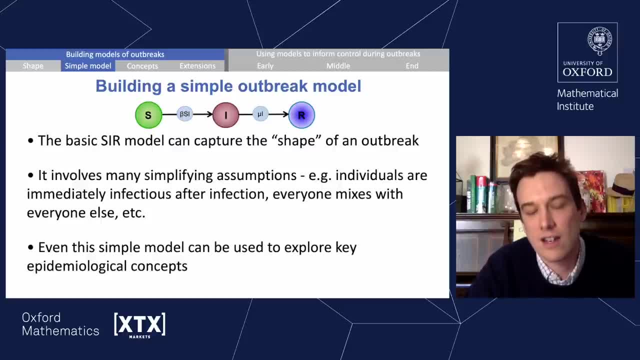 is infectious and starts infecting other individuals. That's clearly not something that's true in reality. There's an assumption that everyone mixes with everyone else. There are lots of different assumptions of this very basic outbreak model. that may not be realistic, but what I'm going to come back to later is how we can extend this basic infectious. 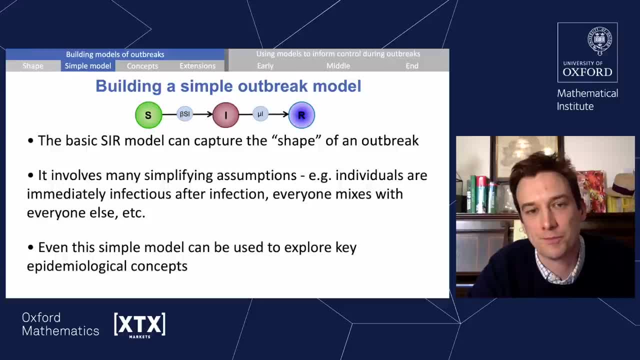 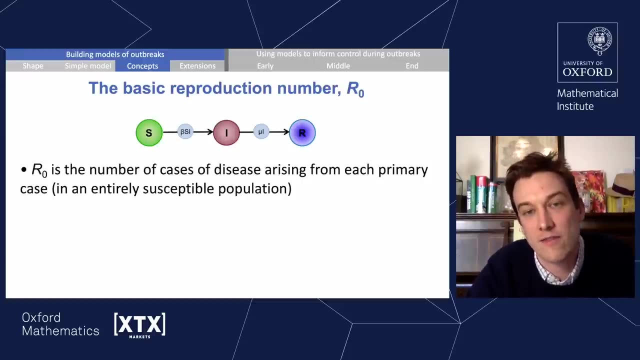 disease outbreak model to include additional realism. Even this simple model, though, So even this SIR model, can be used to explore different epidemiological concepts. So that's what I'm going to do now. The first concept that I'm going to talk about is that of the basic reproduction number. 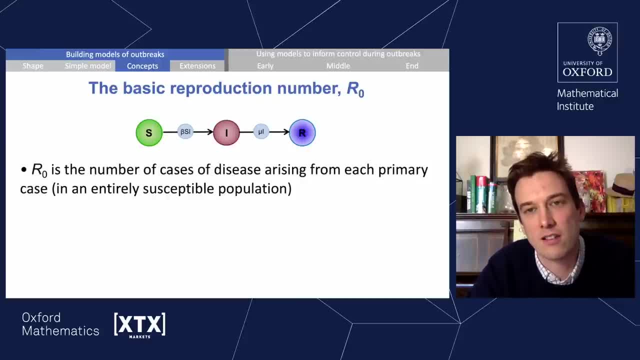 or R0.. This is a quantity that policymakers have been talking about a lot during the ongoing COVID-19 outbreak. So what is the reproduction number R0?? R0 is the number of cases of disease arising from each primary case. So in other words, it's a measure of if I contract an infection. it's a measure of. 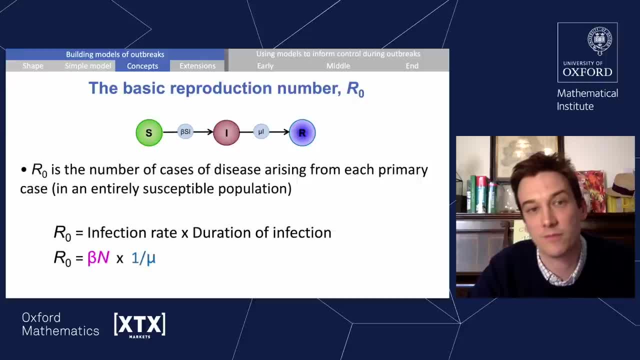 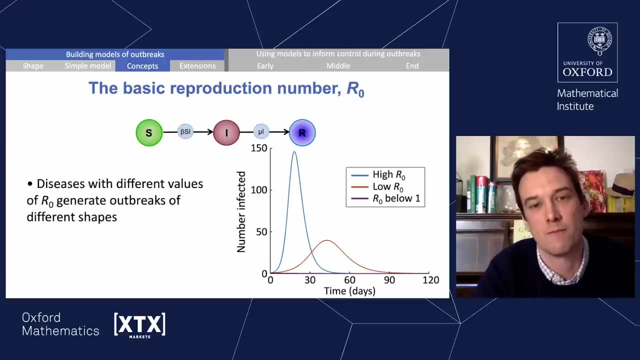 the number of people that I'm likely to go on and infect. You can calculate R0 by simply taking the infection rate and multiplying it by how long an infected individual is infectious, for That's how you go about calculating the basic reproduction number, And diseases that have very different values of the reproduction number generate outbreaks. 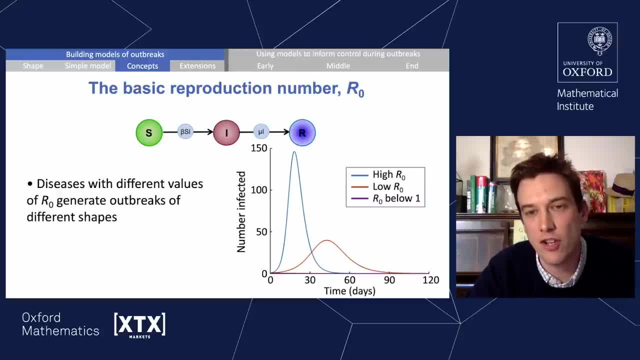 with very different shapes. So, for example, if you look in the bottom right, what you can see is the results of an outbreak with very high R0, in blue. So what you can see is that the disease sweeps through the population very quickly. 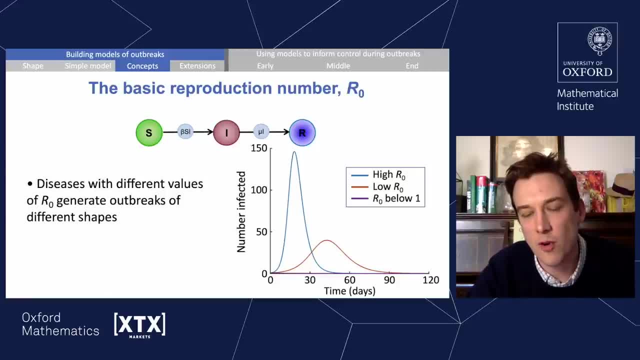 You have large numbers of infections, Whereas if R0 is lower, like the red, then you have a much lower peak and the disease sweeps through the population a lot more slowly. If R0 is down below that, then it's a much lower peak. 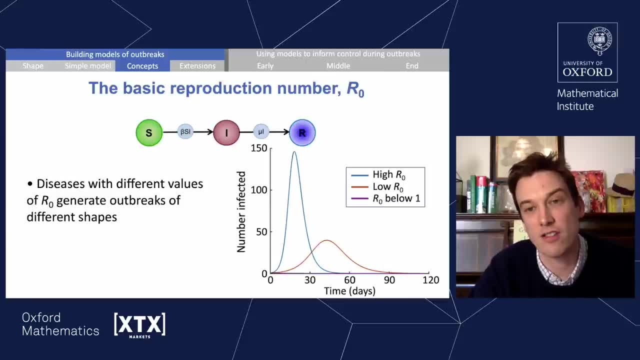 And it's a much lower peak one. well, that means remember that r0 is the number of infections caused by each infectious individual. if r0 is below one, then on average, each infected individual will go on and infect fewer than one other individuals. so, in other words, i'm likely to go on and infect fewer than one person, and so then, 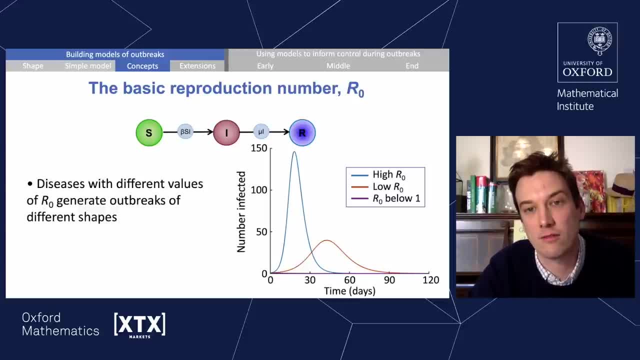 what you see is you see that the disease doesn't spread widely in the population. so then you see something that looks a bit like the purple. it's actually very difficult even to see it in this graph here. but you put in your first infected host. r0 is less than one, and so the outbreak. 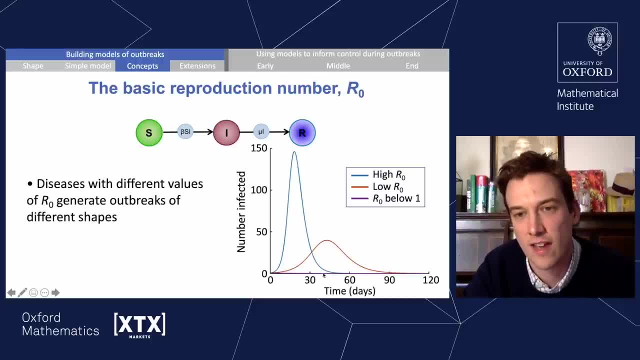 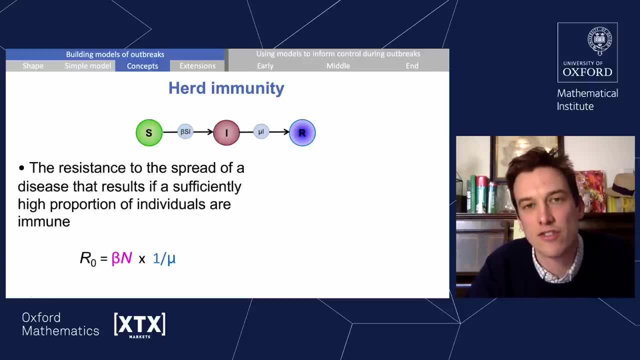 simply fades out. there's a purple line running along the x-axis just here. okay, so another concept that you'll have heard about during this outbreak is the concept of herd immunity. so what is herd immunity? well, it's the resistance to the spread of a disease that results if a sufficiently high proportion of individuals in the population are immune. 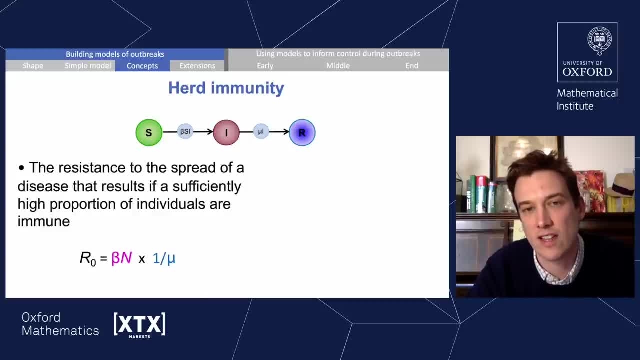 so you can see that the disease is spread widely in the population. so you can see that the disease is spread widely in the population. so you can see that the disease is spread widely in the population. so, in other words, maybe you've got a disease which has been around before and it's infected. 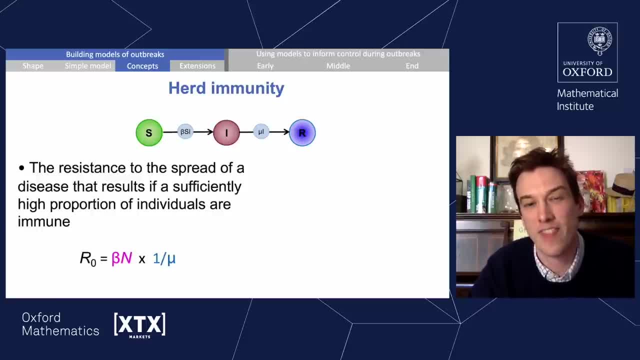 lots of people and those individuals have become immune. well then, that creates resistance to the spread of disease when it reappears in the population. we can actually see how herd immunity works by looking at the effects on r0. so r0, remember, was the product of an infection rate term. 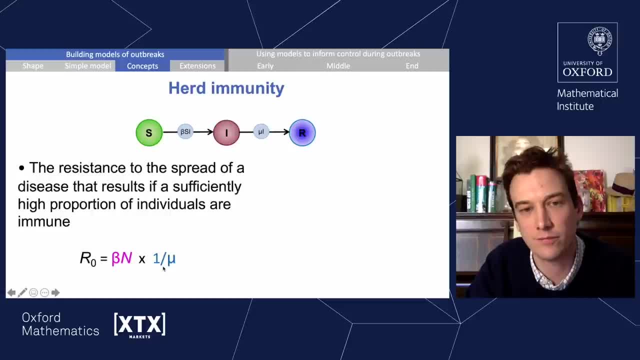 and the duration of infection term, which is this term here. well, the infection rate term is equal to beta times by n, and in this equation n represents the number of susceptible individuals, so the number of individuals that are available to be infected. so if there's a high amount of immunity in the 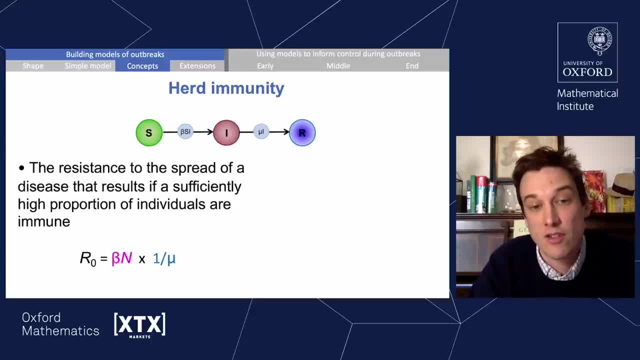 population. what that does is it reduces the number of individuals that are available to be infected, so, in other words, it reduces n, and so if n is reduced, well, then that means that the basic reproduction number r0 is also reduced because of this formula here, and so what we can do then is we can look at those graphs again in the context of immunity. 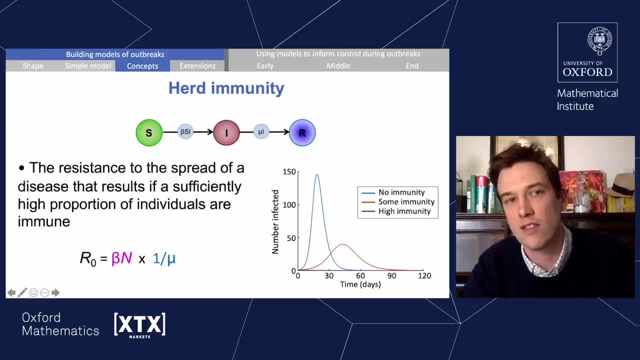 well, if there's no immunity at all, then r0 is high, and so you get an outbreak that looks a little bit like the blue curve. if there's some immunity in the system, though- if n reduces r0 effectively, then there's some immunity in the system, and you instead see an outbreak that looks. 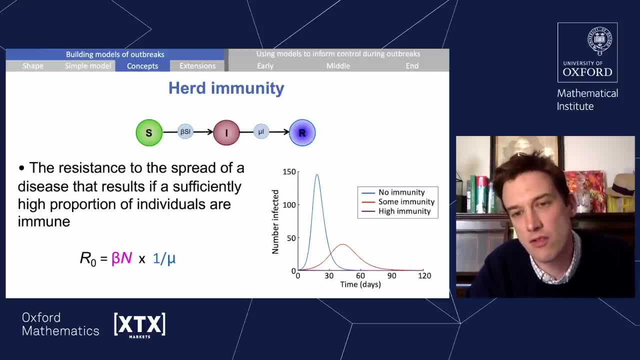 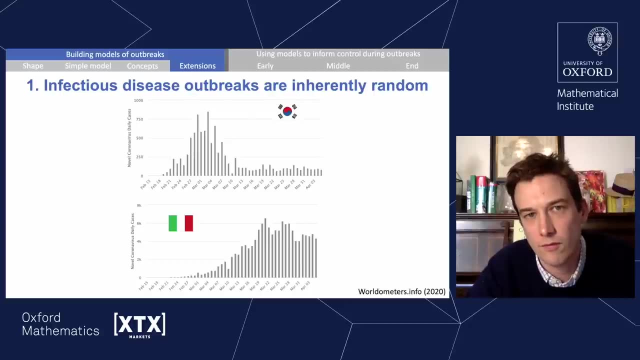 a little bit like the red, and if lots of individuals are immune then you instead see outbreak that looks a little bit like the purple. So again, immunity being in the system significantly changes the dynamics of an infectious disease outbreak. Okay, so we've talked now about a very basic epidemiological model, the SIR model. 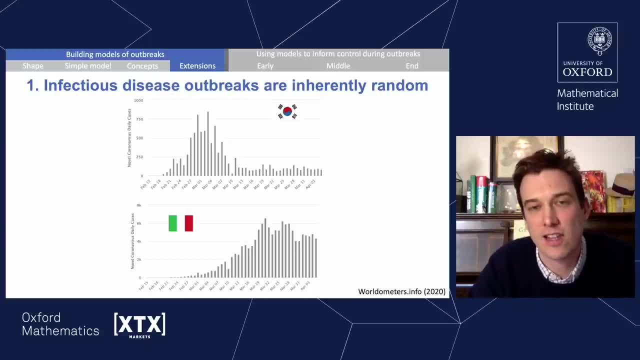 and we've talked about a few concepts relating to infectious disease outbreaks, so concepts like the basic reproduction number and the concept of herd immunity. What I'm going to go on and do now is talk about how we can extend the basic SIR model, and these extensions are ones that are: 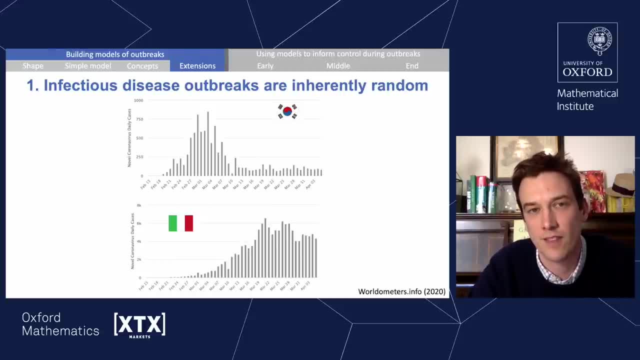 done commonly by infectious disease outbreak modelers. So the first extension is to note that infectious disease outbreaks are inherently random. So, in other words, all of the curves that we've seen so far for the number of infected individuals through time have been these very 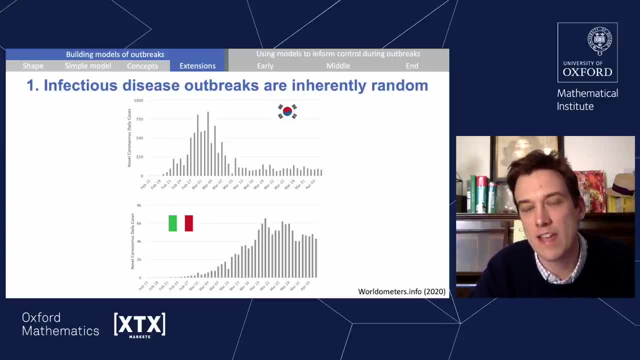 smooth curves right. The numbers of cases went up, it peaks and then it comes back down again, and it does so in a very smooth fashion. But real infectious disease outbreak data just doesn't look like that. So here are a couple of. 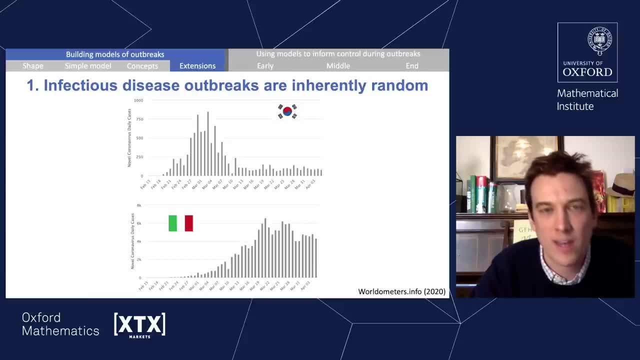 examples. So what we have at the top is we have the number of new coronavirus cases every day in South Korea since February the 15th, And what you can see is that we get the general overall shape of the outbreak. the numbers of cases goes up, it peaks and then it comes back down again. 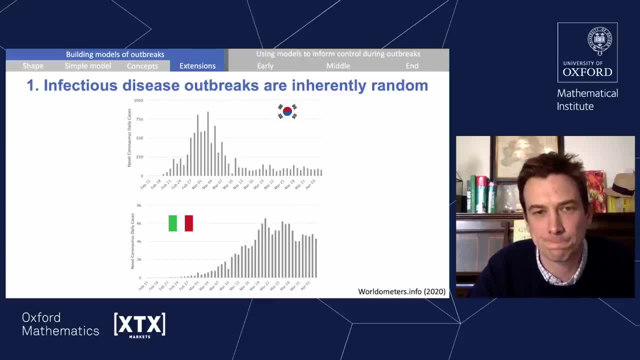 in this particular wave of the outbreak. But what it doesn't do is it doesn't do that in a really smooth fashion. The numbers of cases kind of jags around a little bit. Similarly, if we look at the bottom- so this is data from Italy- we see not a complete wave of the outbreak, but we see 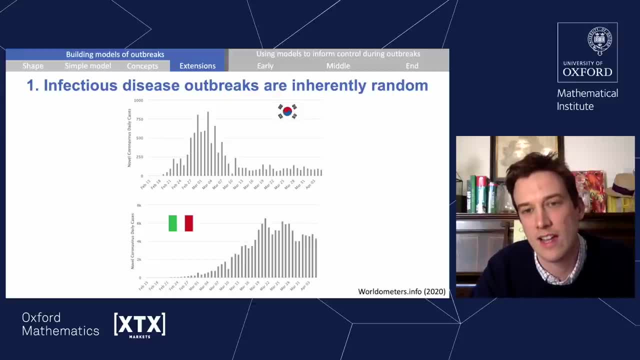 again a similar looking pattern where the numbers of cases goes up, it then looks to peak and then it looks like it's starting to come back down again. But again it does it by sort of jagging around a little bit, not like the smooth curves that we've seen so far for the SIR model. 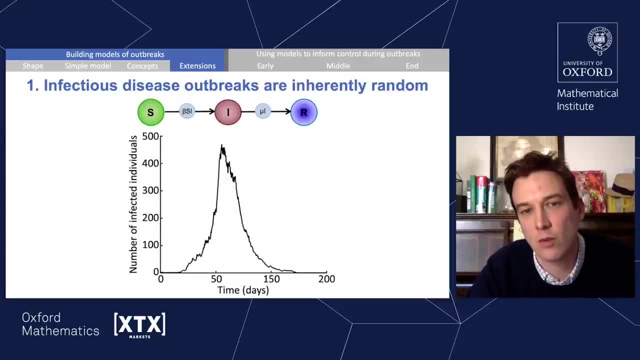 So what we can do is we can do a little bit of a simulation of an infectious disease outbreak by using what's called stochastic models. So the idea of a stochastic model is that an infectious disease outbreak isn't simply a deterministic process, Instead what happens. so, if you want, 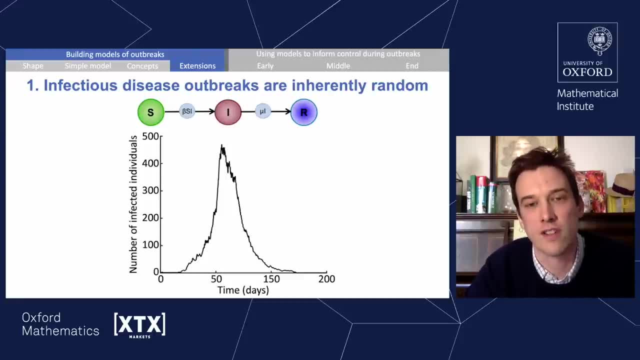 to simulate a stochastic SIR model is: you can simply flip a coin lots and lots of times And then, according to the results of each coin flip, you can either generate a new infection, so a new disease, or you can make one of your infected individuals recover and become immune And just. 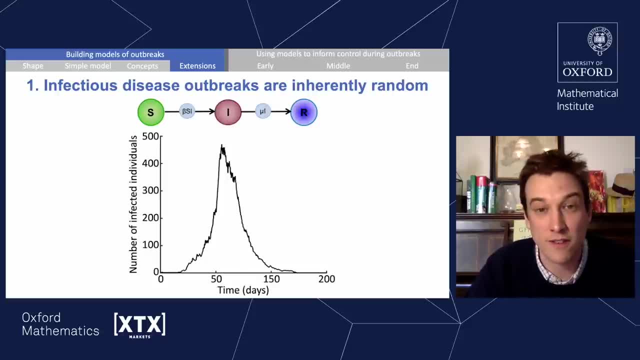 to be clear when we're flipping this coin lots and lots of times, this isn't a fair coin. It's not 50-50, whether or not there's an infection event or a recovery event. Instead, the coin is weighted, and it's weighted according to the number of susceptible individuals and the number 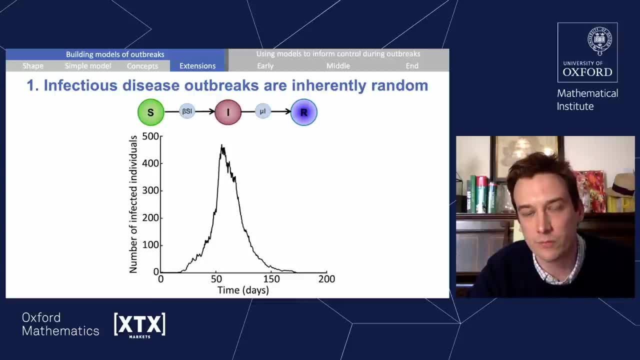 of infectious individuals there are in the population at that time. So, as an example, if you imagine that there are lots of healthy individuals in the population at that time and there are a population at the moment, well, that means that there are lots of targets for infection. So you'd. 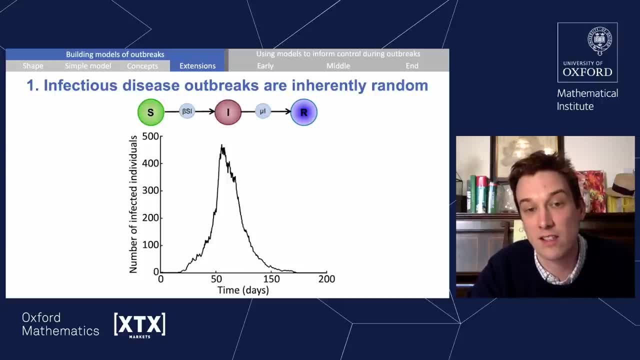 expect the chance that the next event is an infection event to be high, because there are lots of potential individuals that could be infected, And so you'd weight the coin when the number of susceptible individuals is high, so that the chance that the next event is an 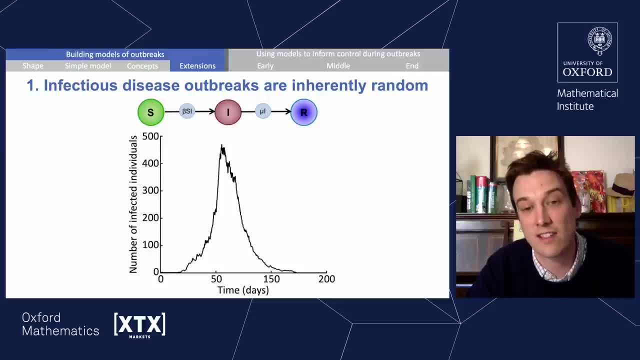 infection event is high compared to the chance that the next event is a recovery event. So what we do is we flip a coin lots and lots of times And, according to the results of each coin flip, we change the state of the system. So this is one example. Again, this is nothing to do with. 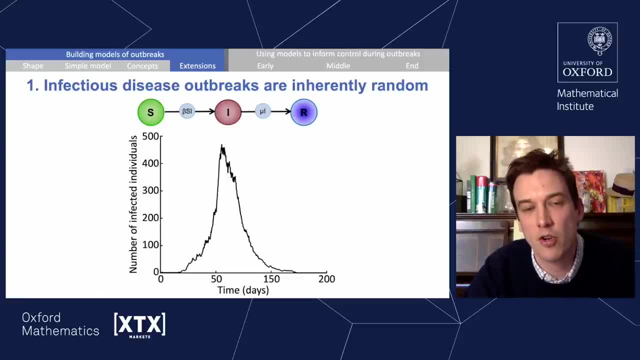 COVID-19,, but it's just to show the idea. So we flip a coin lots and lots of times and we see this graph- the number of infected individuals. through time. We can then repeat that if we want to. So we can generate a new simulation of an infectious disease outbreak by simply flipping. 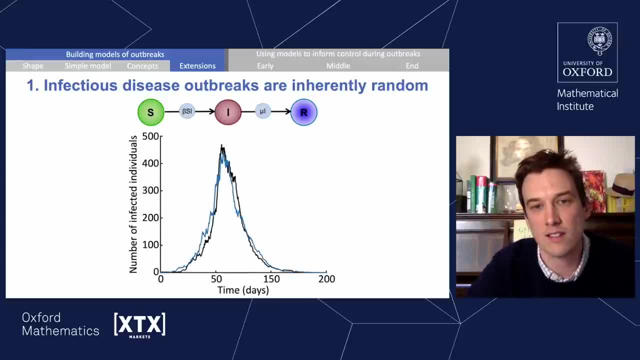 a coin lots and lots of times again. And if we do that, then in a second simulation under absolutely identical conditions, we can then generate a new simulation of an infectious disease outbreak. by simply flipping a coin lots and lots of times, We might see an outbreak that instead looks like. 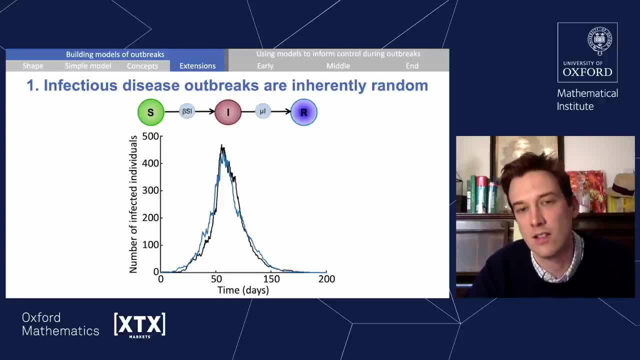 the blue curve there. So qualitatively, the blue curve and the black curve are pretty much identical, The only difference- so the reason that they don't look exactly the same- is that we've got a slightly different sequence of coin flips. We've got a slightly different sequence of 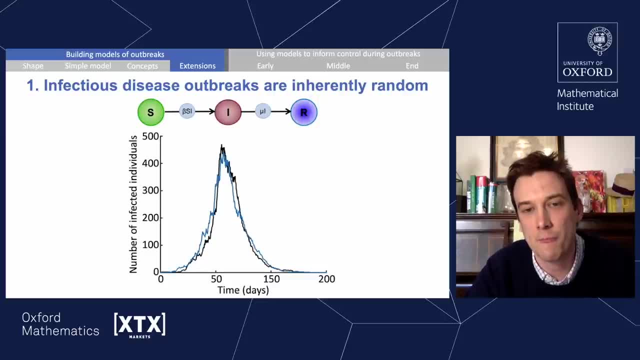 infection and recovery events. So then, what we can do, if we want to, is we can actually run another simulation again under absolutely identical conditions. So, again, we generate a sequence of coin flips, And if we do that, we might instead see something that looks a little bit like the red. 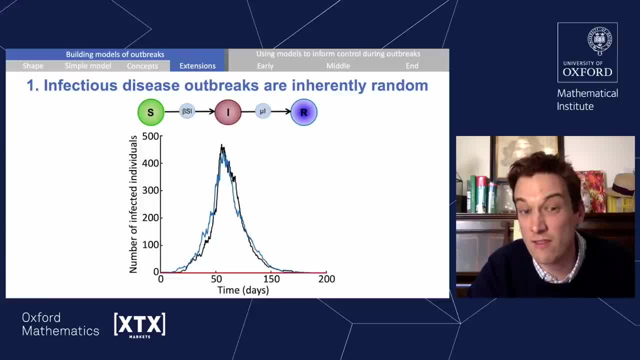 line there. So what's happened this time is we've started with one infected individual. We've generated a sequence of coin flips, but the first coin flip has indicated that the one infected individual has recovered without infecting anyone else. And because they've recovered without 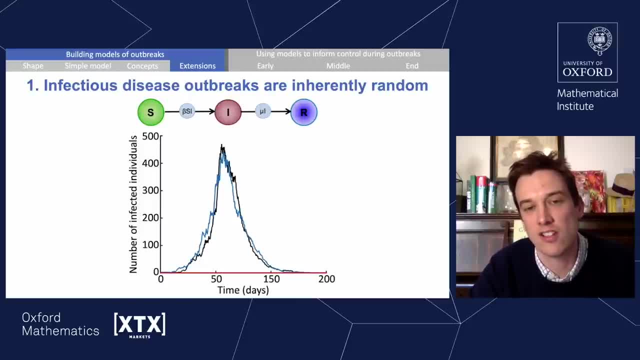 infecting anyone else. the disease isn't in the population anymore And so the outbreak simply fades out. So by including this randomness in the sequence we can then generate a sequence of coin flips in the model. Then you can get very different qualitative behaviour each time you run a. 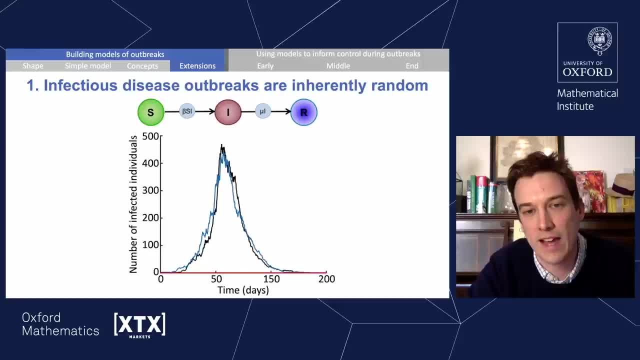 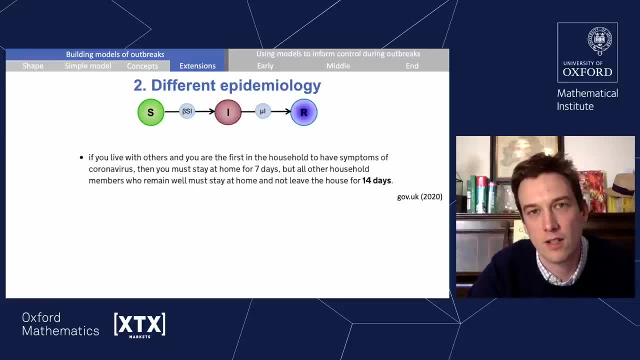 simulation. You can either get a big outbreak, like the blue or the black, or you can get a very small outbreak, like the red. Okay, So another thing you can do to extend the basic SIR model is you can include all sorts of different infectious disease epidemiology. So I'm going. 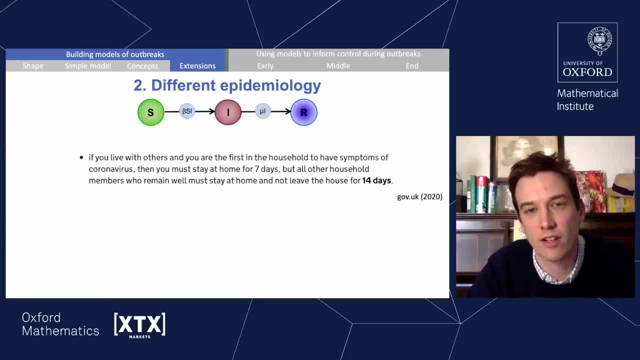 to talk about one particular example in the context of some of the current government guidance for COVID-19.. So the current government guidance for COVID-19 is that if you live with others and you're the first in your household to have symptoms of a coronavirus infection, then you should stay. at home for seven days. All the other members of your household, on the other hand, must stay at home for 14 days. So what you can see there is that the other members of your household- if you're the infected one initially, the other members of your household may not even be carrying the virus. 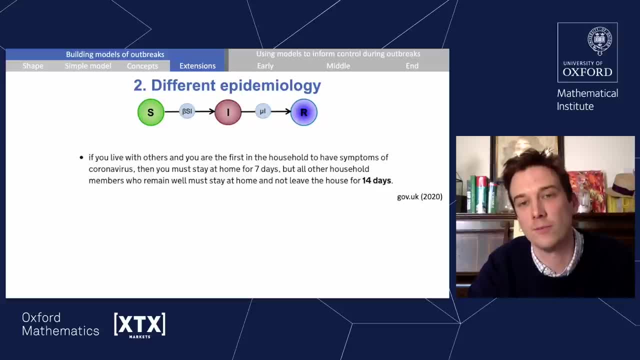 yet they're expected to stay at home for 14 days, So the other members of your household may not even stay at home for longer than you are. But this rule in fact makes complete sense, And the reason for that is that there's a delay between an individual becoming infected and an individual. 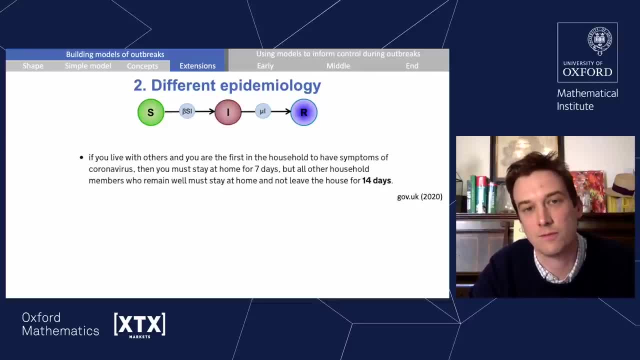 showing symptoms and starting to infect other individuals. So what that means is that, well, suppose that I get the infection. Well, let's suppose that I'm symptomatic, let's say for seven days. Within that seven days, then I might go and infect someone else in my household and they may. only show symptoms and start infecting other people. So I might go and infect someone else in my household and start infecting other individuals in the second set of seven days. So that's why it's very important that other household members stay at home for a longer period, for a period of 14. 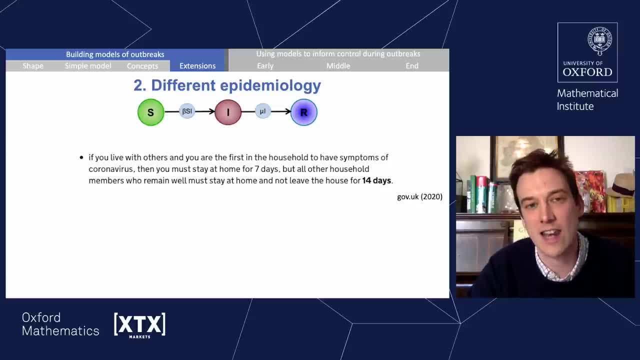 days. So, like I say, the key thing here is that there's a delay between an individual becoming infected and that individual starting to show symptoms or infect other individuals, And we can include that in the basic SIR model by simply including another class in between being. 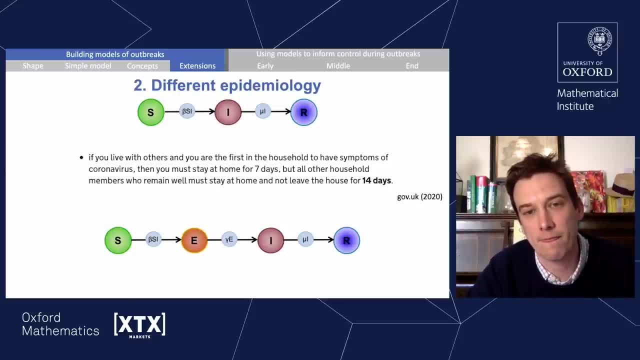 susceptible and being infectious. So, in other words, we can build a model that looks like this one on the screen now, where you have susceptible individuals and after infection they enter this E class, And E class represents individuals that are infected but they're not yet generating new infections, And then only some. 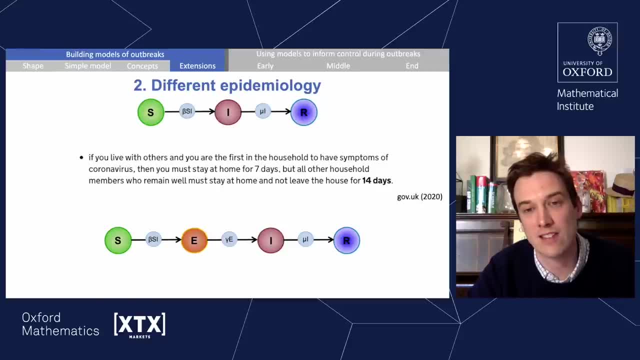 time later do infected individuals become infectious and enter the I class And then eventually, after they've been infectious, they recover and enter the R class. So this model here includes this sort of additional bit of epidemiology, the fact that there's a 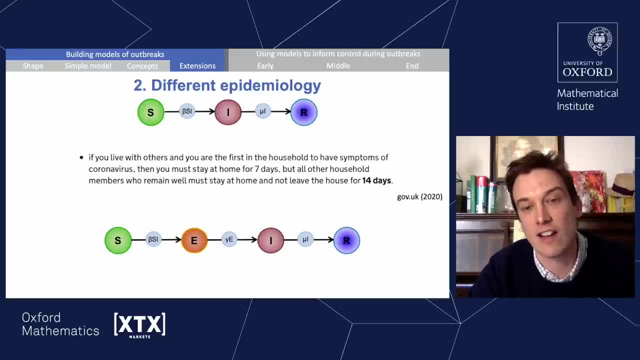 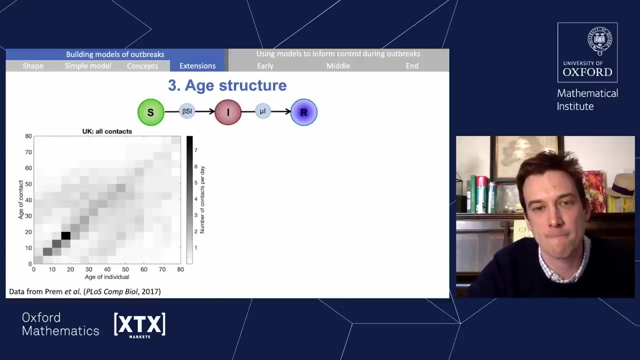 delay between being infected and then starting to generate new infections. And you can include other types of epidemiology in compartmental models in a similar way. You can simply introduce new compartments into the model to represent different aspects of the underlying epidemiology. So another thing. 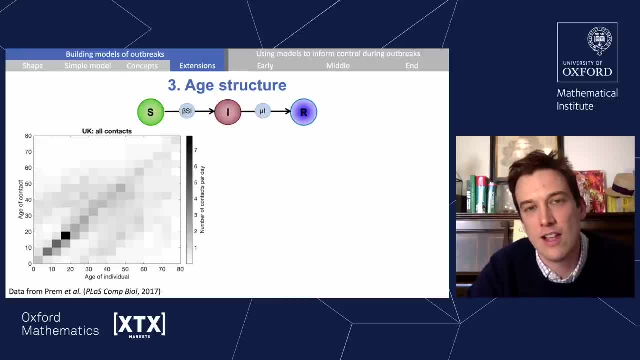 that you might like to include in an infectious disease outbreak model is the idea that individuals of different ages contact other individuals at different rates. So here's an example. So this is a graph that shows this quite clearly. I think This is data from a paper by Prem et al in PLOS: Computational Biology and 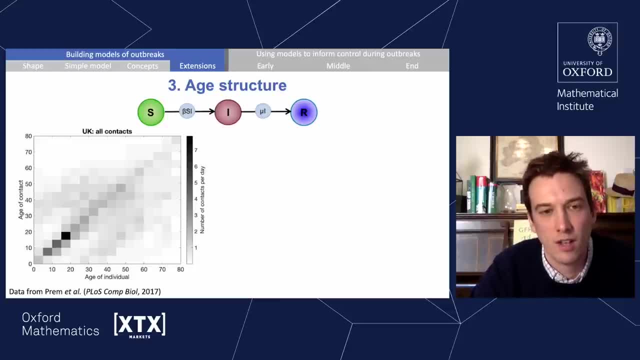 this graph was created by one of my PhD students, And what you can see is so: on the x-axis you've got the age of an individual, and then on the y-axis, you've got ages of the individuals contacted by the individual, And then the colour in the graph represents the number of contacts per. 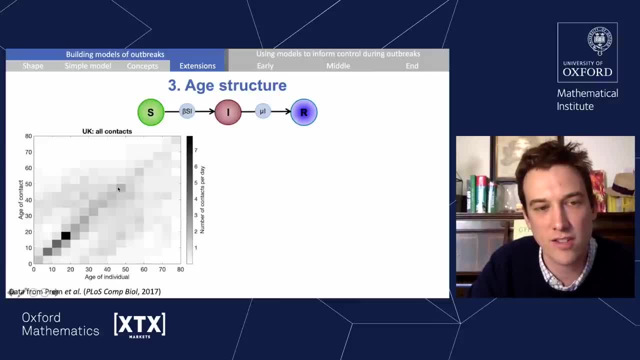 day between individuals of those ages. So what you can see is you can see this diagonal here which is quite dark. So this diagonal represents individuals on the x-axis contacting individuals on the y-axis, and what you can see is that, because it's this diagonal that's quite dark, that means that it's reasonably 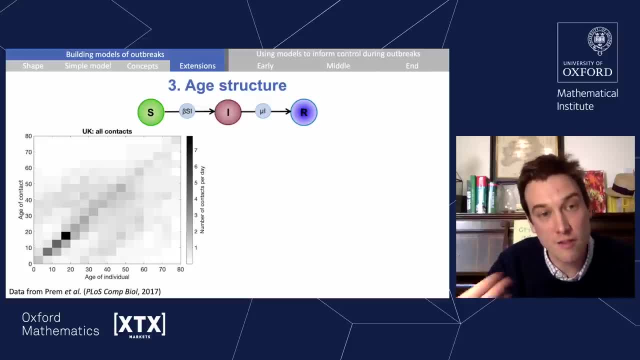 likely that an individual of a certain age will contact other individuals at the same age. You can also see some other kind of dark areas as well on this, on this particular graph. So here there are some dark areas up here and there are also some dark areas down here. This dark area down here represents an adult. 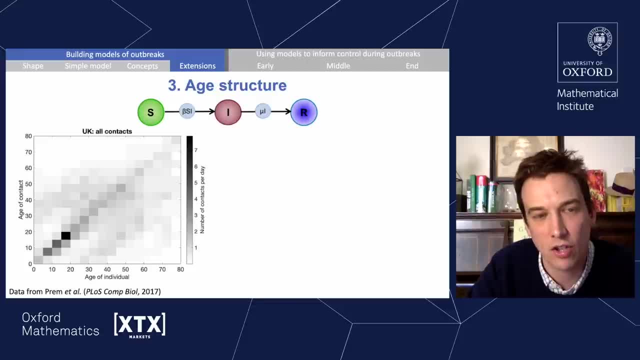 that's roughly of an age of a parent contacting someone that's the age of a child. So this particular streak represents parents contacting their children. So this dark area up here represents individuals that are the age of a child contacting individuals that are the age of an adult. So this particular area up 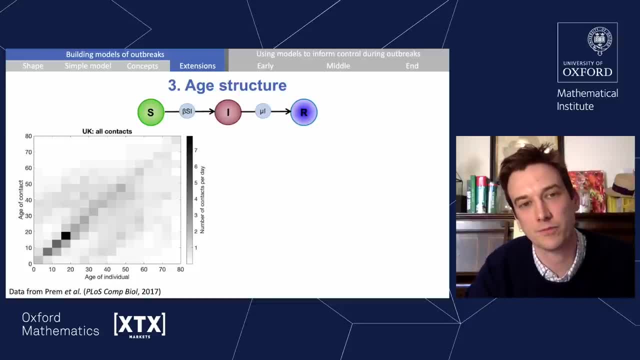 here represents children contacting their parents. You can really clearly see that there's some very strict age structure in who contacts whom within a population. You can also look at contacts in different settings, so that's what we have here. So this middle graph here represents home contacts, and you can 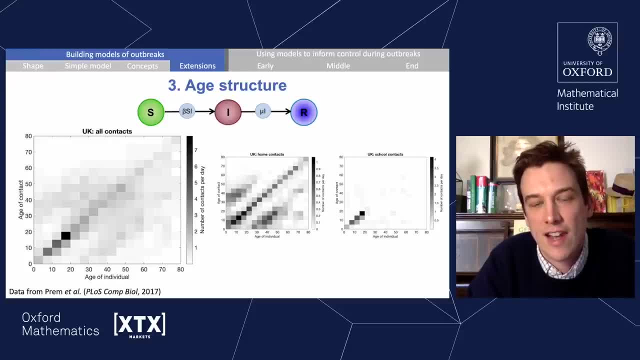 see very similar patterns to the ones that I just described in the left graph. So, in particular, what you can see here is that at home, it's very likely that individuals contact individuals of the same age, and it's also very likely that individuals- so parents contact children and children contact parents. But if you 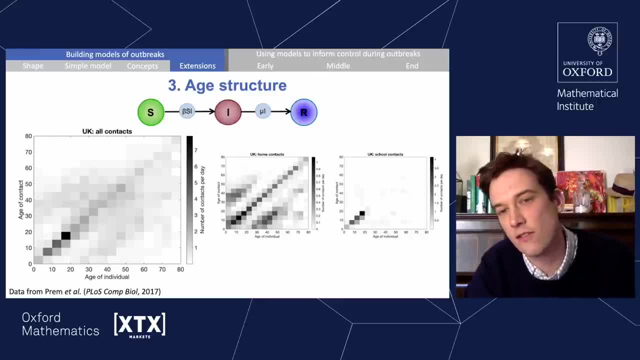 look in another setting, then contacts will look different. So if you look, for example, at the right graph, well, the right graph represents school age contacts and what you see in schools is that the majority of contacts are children contacting individuals of the same age. So this kind of age structure. 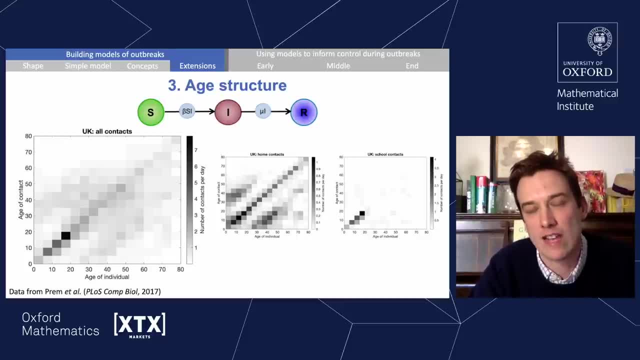 wasn't represented in the basic SIR model that we looked at earlier. The assumption in the SIR model was that everyone of every age contacts other individuals at a kind of constant rate, Whereas the data that I've shown on this particular slide here shows that that clearly isn't the case. But age structure: 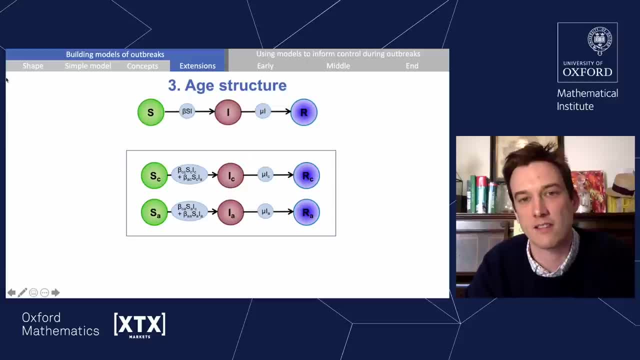 can very straightforwardly be included in a model like the SIR model. So here's one way to do it. So, in this particular model that I'm showing here, we just have individuals of two ages, So we just have children and we have adults. This approach, though, the approach I'm showing you here, can 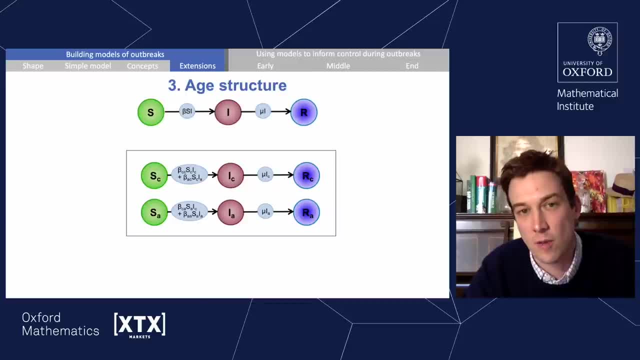 easily be extended to any number of age groups you want. So, in particular, the data on the previous slide can all be incorporated in an SIR type model if we want to do that. But here, in this very basic extension, we have individuals that are children and adults, and what we essentially have is 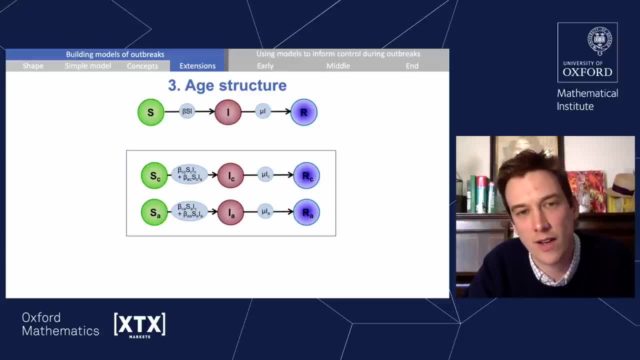 we have an SIR model for children. So that's this one on the top where you have susceptible children, infected children and recovered and immune children, And then we also have an SIR model on the bottom for adults. So again we've got susceptible adults, infected adults and recovered and immune adults. 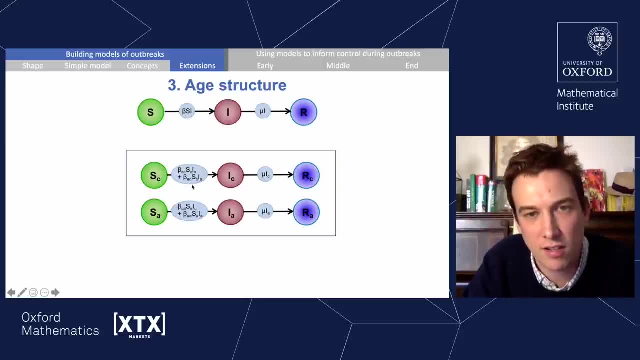 And something to notice here is that if we look at the infection rates term- which are these terms in here- the infection rates depend on: so this is the rate at which children become infected. that depends on the rate at which children infect other children. this beta CC term. 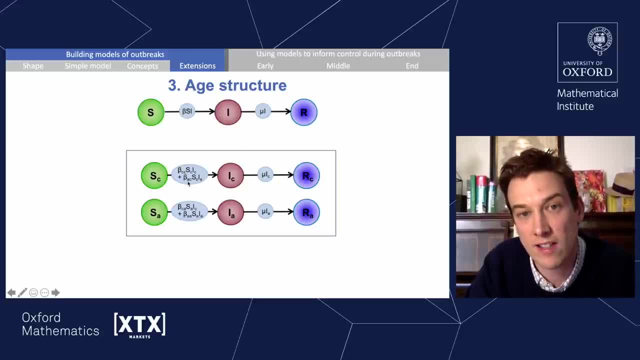 And it also depends on the rate at which adults infect children. so it depends on this beta AC term. So if children have lots of contacts with other children, then you might expect that the beta CC term, the infection rate between children would be high, and so then the rate at which 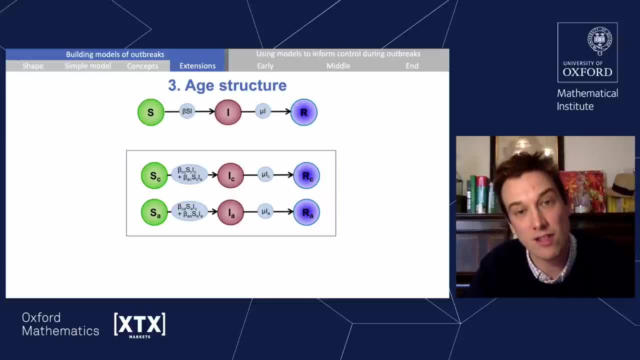 children become infected will also be high. Similarly, if adults have a lot of contact with other children, well then the beta AC term would be high, because the number of contacts is high, then the infection rate is also high, And so then again, children would be infected at a very high rate. So in other words, the 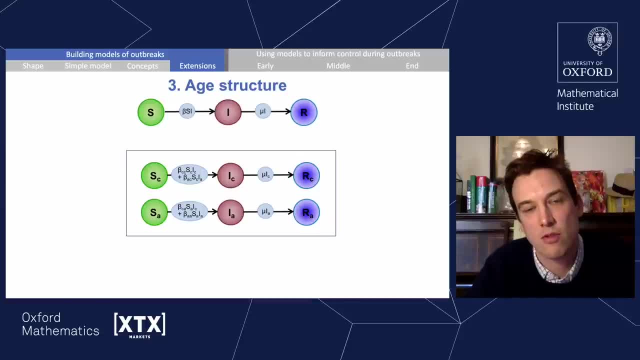 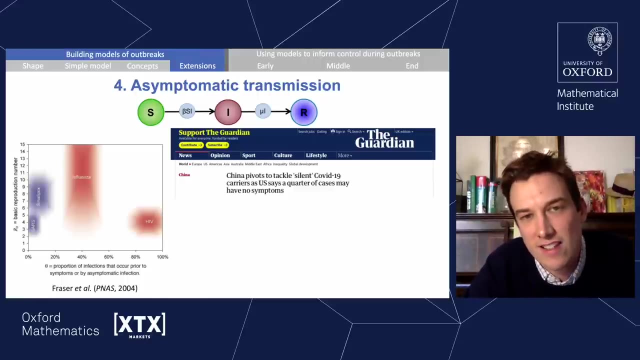 data from the previous slide, the data on the numbers of contacts between individuals of different ages, is included in this model via the various different beta terms, so via the various different infection rate terms. Another thing that we can include, another extension to the basic SIR model, is to: 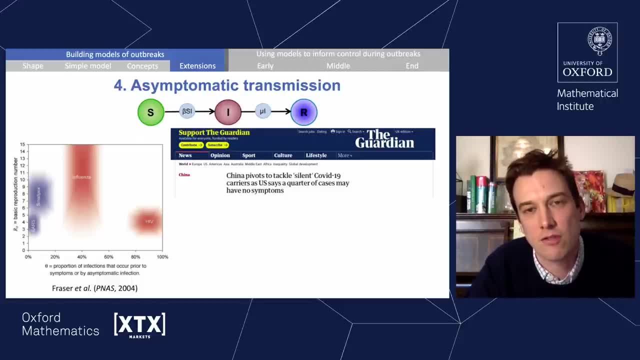 include asymptomatic transmission or transmission from individuals with very few symptoms. This has been something that's been talked about a lot in the context of COVID-19.. So for COVID-19, infected individuals could have any of a wide spectrum of symptoms, So an individual could have very clear. 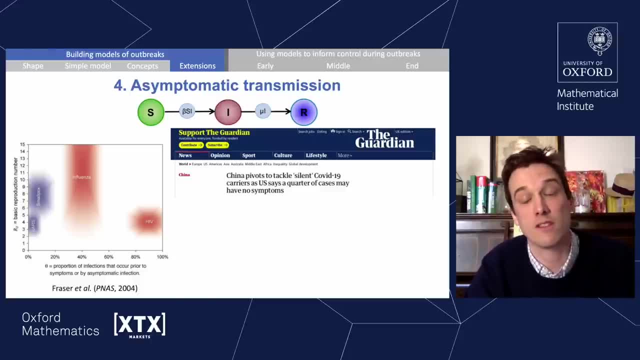 symptoms, but it's also possible that they have very few symptoms. And if the infected individual has very few symptoms, then that makes the outbreak difficult to control, because an individual can be spreading the virus without even knowing that they're doing so. With that in mind, 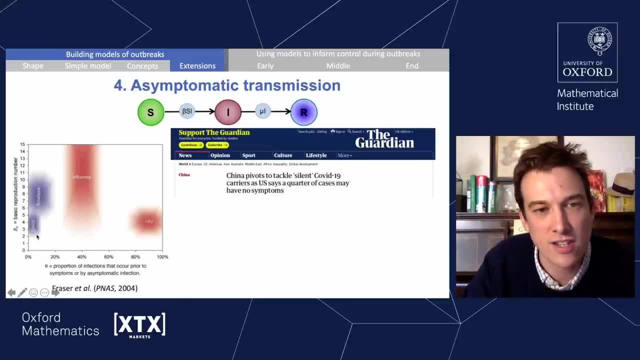 I just want to show you this figure here on the left. So this is a figure from a paper by Christoph Fraser in PNAS in 2004.. Christoph Fraser is now based in Oxford, and what you can see is: if so, the value on the x-axis is the. 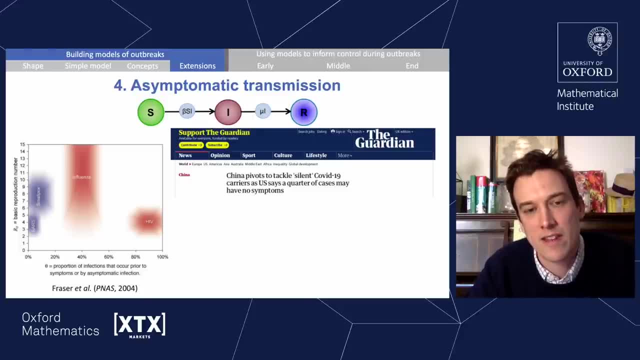 proportion of new infections that arise from the spread of COVID-19, and the number of new infections that arise from individuals that have very few symptoms. So it occurs from individuals either prior to them developing symptoms or from individuals that never develop symptoms, And what you can see is that 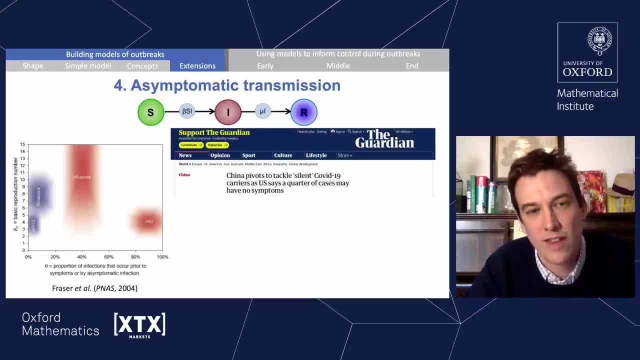 this SARS cluster here. this SARS cluster is on the left hand side of this graph, So what that means is that almost all SARS infections were from individuals that were displaying clear symptoms. So that's very important, because what it means is so. 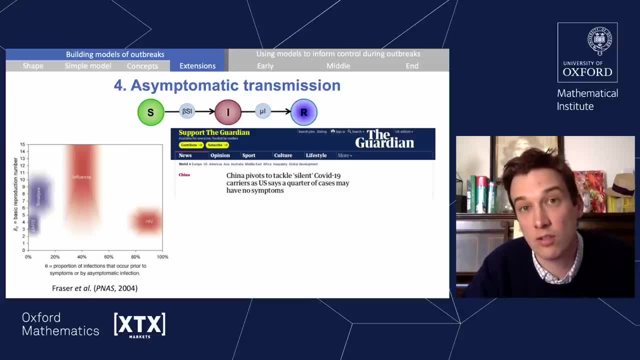 we can actually go out and actually find individuals that are displaying clear symptoms. So, in order to control the outbreak of SARS in 2003,, what could be done is we could go out and actually find individuals that are displaying clear symptoms. We can make sure that we isolate those individuals to make sure. 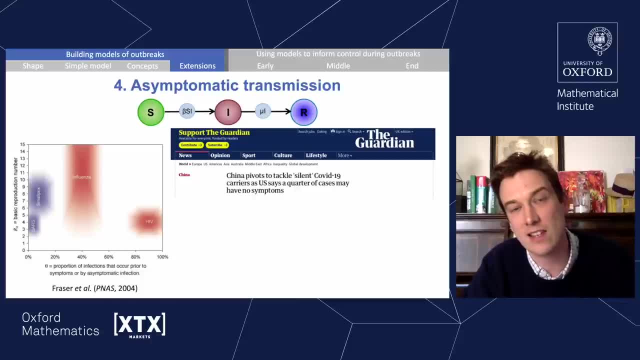 that those individuals with clear symptoms don't transmit to anyone else, And so by isolating individuals with clear symptoms, you could actually bring the outbreak under control. That's something that's unlikely to be possible, because it isn't the case that the only infections out there are driven by 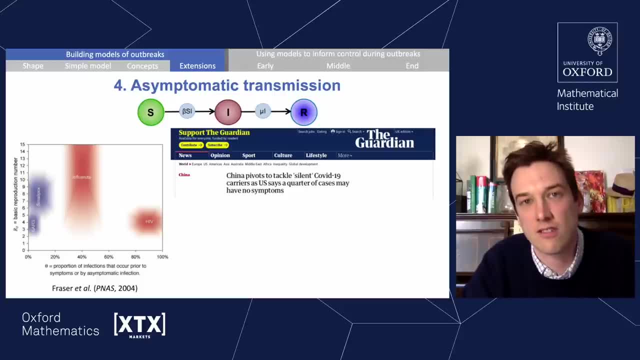 individuals with clear symptoms. So, in fact, a large number of infections are driven by individuals who don't have clear symptoms, And so that means that we have to introduce control strategies that don't only target symptomatic hosts, but also target all of us, because we might be spreading the virus without knowing that we're. 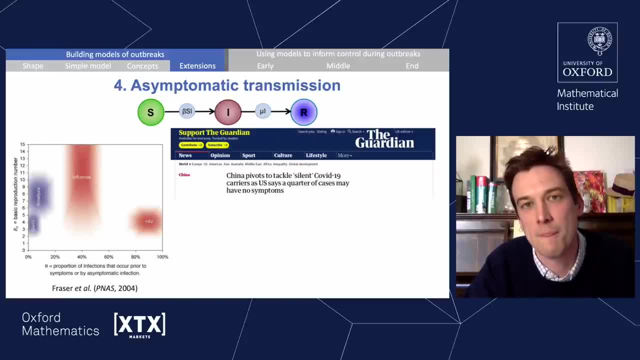 doing so. That's why we need to implement measures like social distancing that have a huge impact on everybody. So this idea, then, about asymptomatic transmission: well, that can be included in a model like the SIR model, And so here's an example. So, basically, this is exactly the same as the SIR model, The only thing? 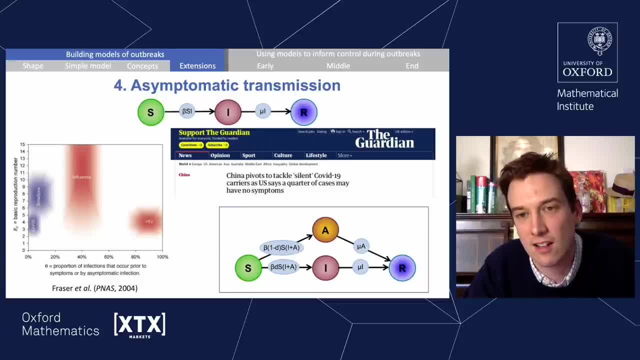 that I want to point out is that we have this additional class in the model, this A class, and this represents individuals that are infected and are transmitting the underlying disease, but they're not showing any clear symptoms. These are the asymptomatic carriers of the disease. 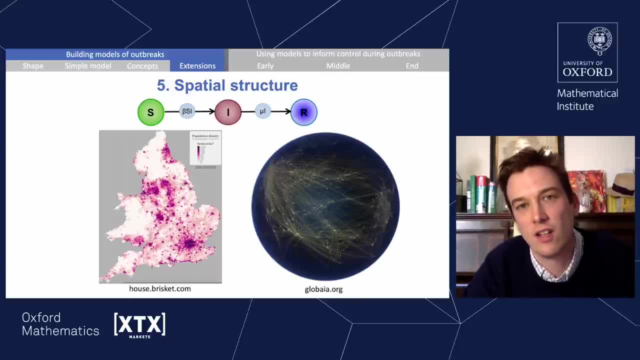 Something else that can be included in the basic compartmental modelling framework is the idea of spatial structure. So here on the left there's a graph which represents the population density throughout England and Wales, And there are two features that I want to point out. The 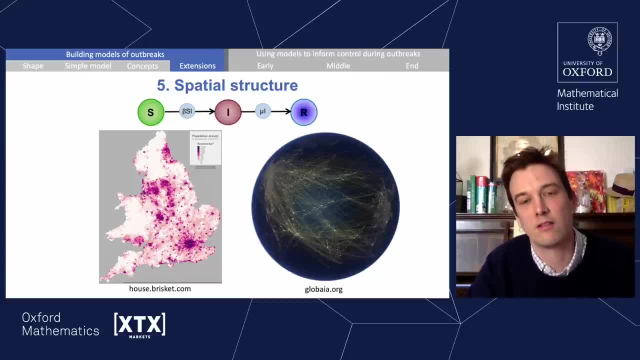 first feature is that the population is very widely spread And actually it's pretty unlikely that if you've got an infected individual on the south coast, let's say that they go on a directly infect someone living in the very north of England. That is very unlikely. Similarly, 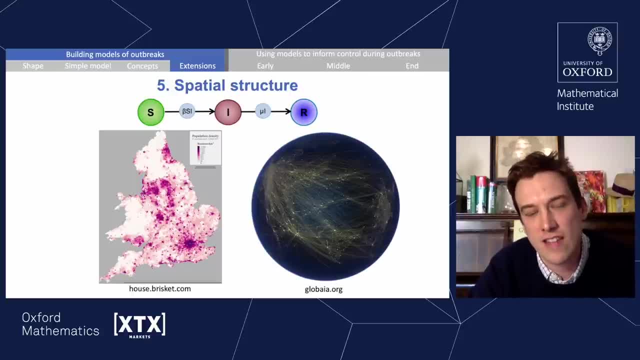 so another thing that you can notice from this graph is that the population density varies substantially throughout the country, And these things can all be included in infectious disease outbreak models like the SIR model. On the right hand side is a graph of air traffic routes over: 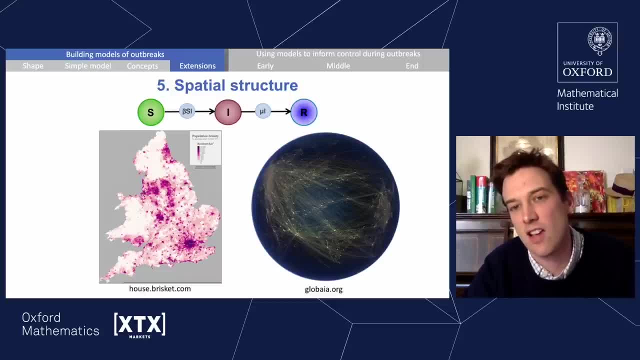 Eurasia, And what you can see here is that some areas are very well connected and other areas are a lot less well connected, And again, that's something that we can include in an SIR type model if we want to, And this is how we do it. So what I'm considering here is: I'm considering a model. 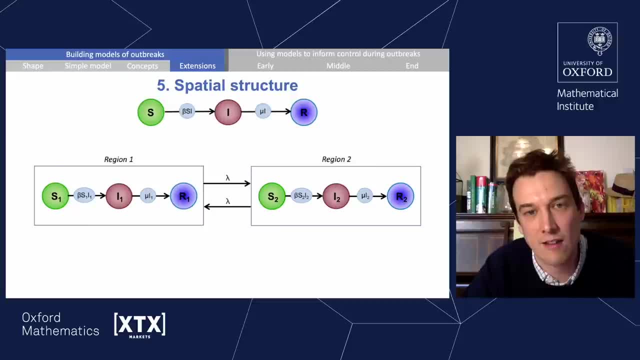 which only has two regions in it, so two spatially distinct areas, But you can extend this idea to any number of regions you want, And so what we have in the first region is we have an SIR model. In the second region, we also have an SIR model And we can include individuals moving. 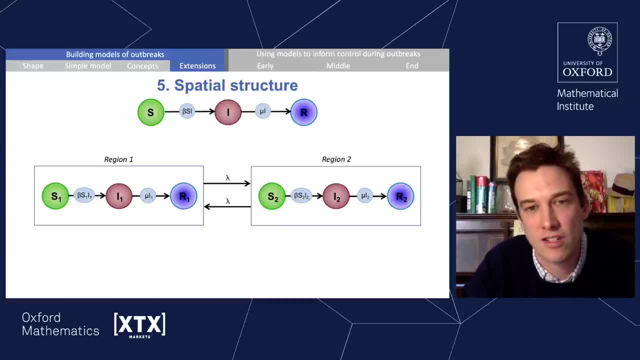 between these two regions. There's some kind of coupling between these two regions at a particular rate, which, in this model, is represented by lambda, And if you have regions, some of which are better connected than others, then you would simply change the value of lambda between two. 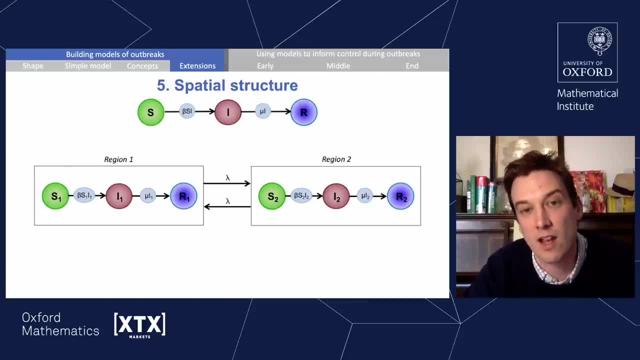 different regions, So a higher value of lambda would represent a better connection between two particular regions. You can include different population densities in these models by simply having different numbers of individuals in total Within each region And in regions that are a long way apart. so you can include that if you want to. 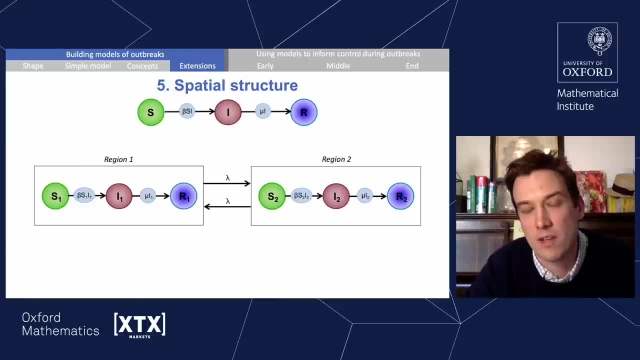 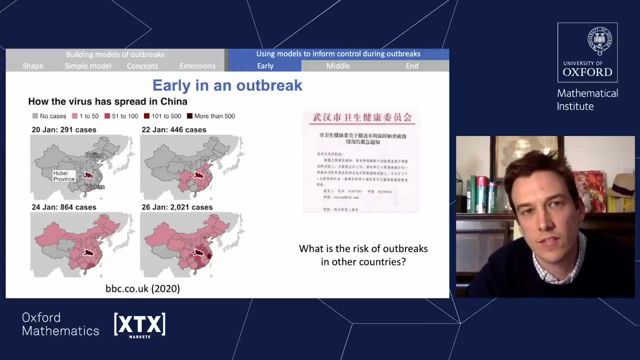 in the model by again assuming a smaller value of lambda, because transmission is perhaps less likely if regions are a long way apart from each other. So that's how, or in fact one of the ways, the spatial structure can be included in a model like the SIR model. So what we've talked about. so 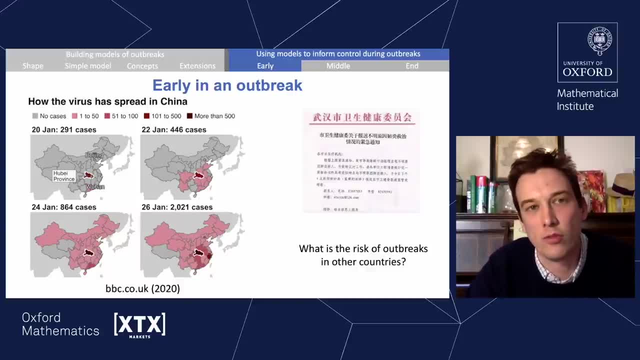 far is. we've talked about how a very basic infectious disease outbreak model can be developed. The SIR model matches the kind of shape of most infectious disease outbreaks. We've talked about various concepts like the reproduction number and like herd immunity, And we've talked about how. 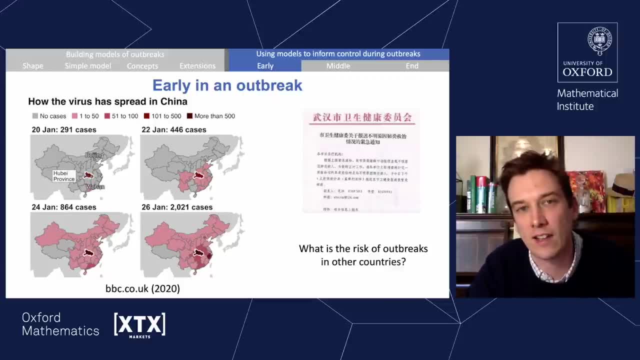 models can be extended from the very basic model I showed you near the beginning to much more complex settings that are much more realistic. What I'm going to talk about now is how models can be used to inform control during outbreaks So clearly. one example of this is the ongoing COVID-19. 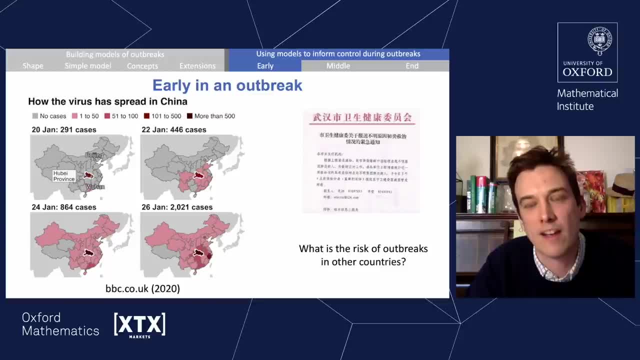 pandemic. So I first heard about this pandemic right back in early January. So I think it was something like the 8th or the 9th of January when I saw the note that's on the right hand side of this figure. So I 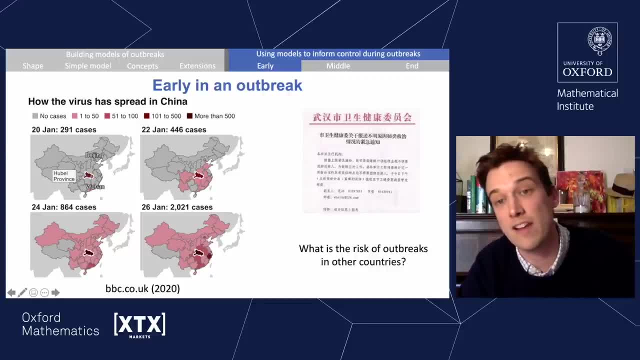 saw this note. it was posted on Twitter and this is a public health notice that was posted in the city of Wuhan in China, And this public health notice says that there have been a number of cases of atypical pneumonia in the city of Wuhan. And the thing that these cases appear to all have in 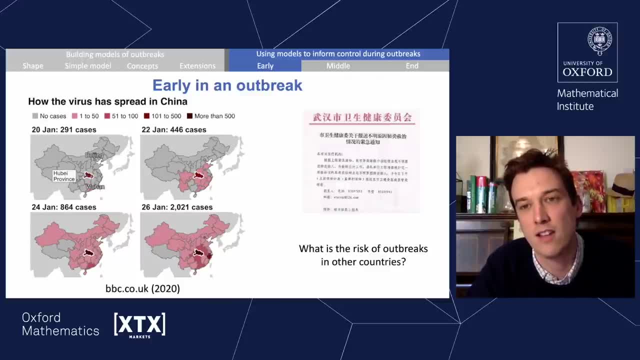 common is travel to the Huanan seafood market in that city, And so one of the first things that I did was I started to go about collecting information about COVID-19. And I started to go about developing mathematical models for this particular outbreak. What we saw as January went. 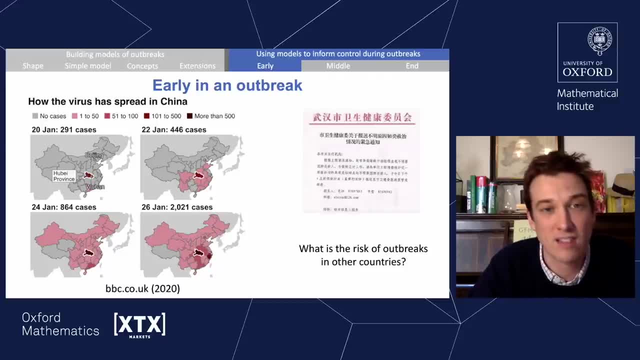 on. so as January this year went on, is that the numbers of cases started to accumulate within China. So on the 20th of January, there were 291 reported cases. Only a couple of cases were reported in China. So on the 20th of January, there were 291 reported cases, Only a couple of cases were. 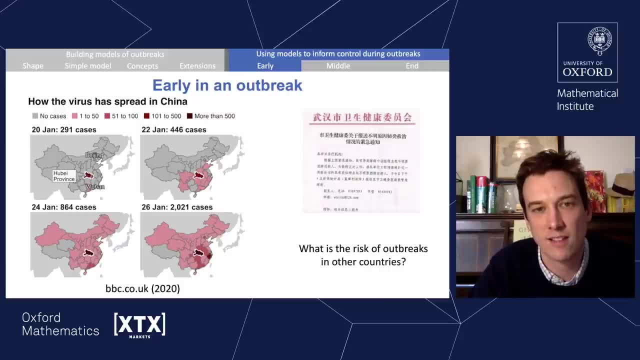 reported in China. So on the 20th of January there were 291 reported cases. Only a couple of cases were reported in China. So on the 20th of January there were 291 reported cases. Only a couple of days later, there were already 446 cases, And by the time we got to the 26th of January, 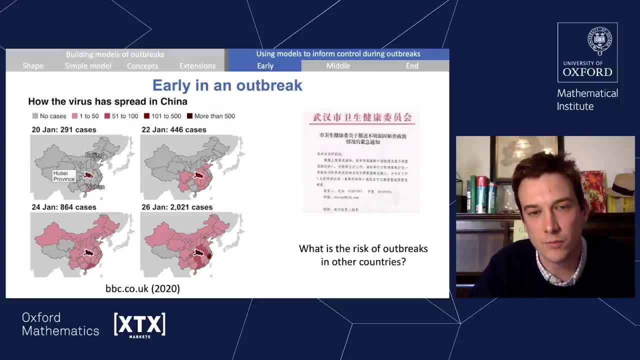 there were over 2000 reported cases, And so the question that I wanted to answer, as the outbreak was spreading within China, is: well, what is the risk of getting outbreaks in other countries? How likely is it we see an outbreak like the outbreak that we're seeing in China, but in the 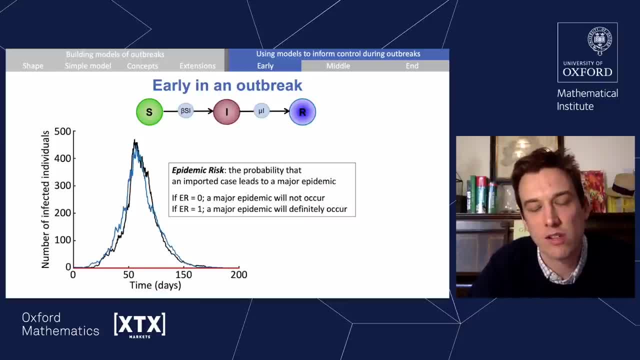 UK And, again, models can be very useful to explore questions like that. So, again, this particular graph is not specifically for COVID-19, but it demonstrates a key epidemiological principle, And that key epidemiological principle is that of the epidemic risk. 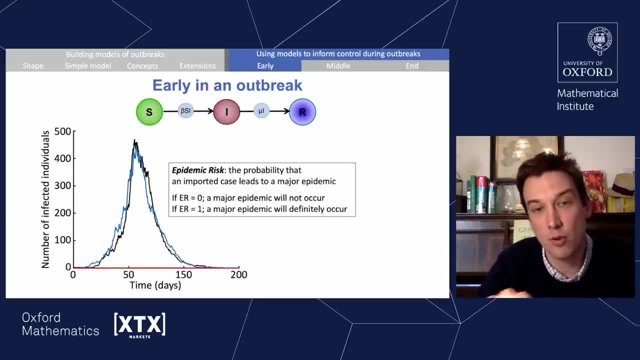 So the epidemic risk. so what is that? So that means every time you get an imported case, it's simply the risk that that imported case in a new location generates a large outbreak there. So do they start chains of transmission that lead on to a large outbreak. The graph: 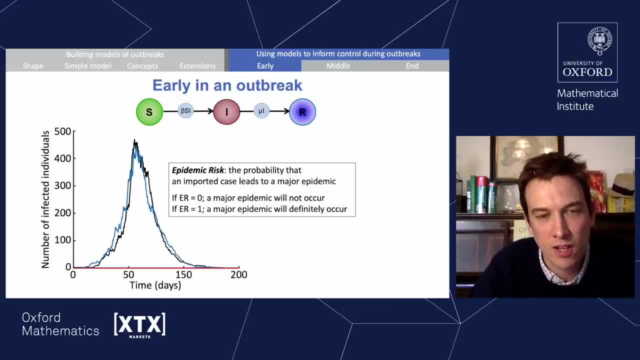 that I'm showing here is the graph that I showed you a bit earlier, And in that graph, what I showed you was that when you run a stochastic epidemic model, you can either see a large outbreak, like the blue or the black, or you can see a small outbreak, like the red. 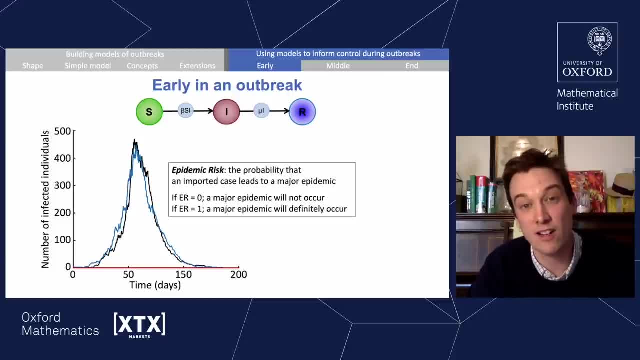 So if the epidemic risk is zero, what that means is that every time you get an imported case, you're not going to get a large outbreak. You're always going to see something that looks like the red and not something that looks like the red, And so you can see that if you run a 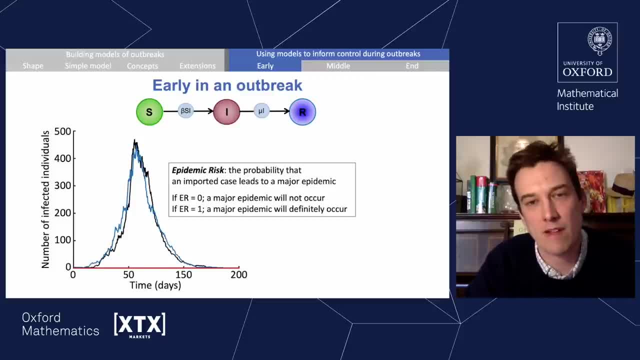 like the blue or the black. If, on the other hand, the epidemic risk is 1,, well then a major epidemic is definitely going to occur. so, in other words, every time you get an imported case, they're going to start chains of transmission that lead to a large outbreak like the blue or the black, rather than a small. 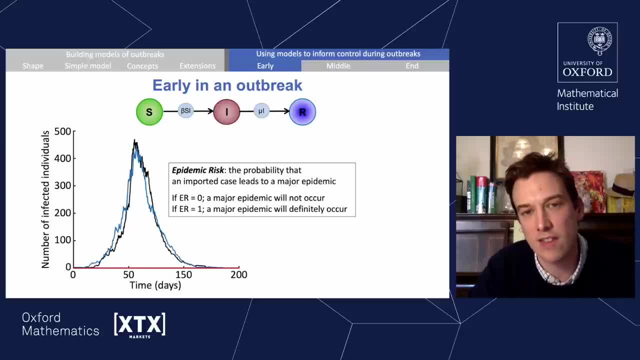 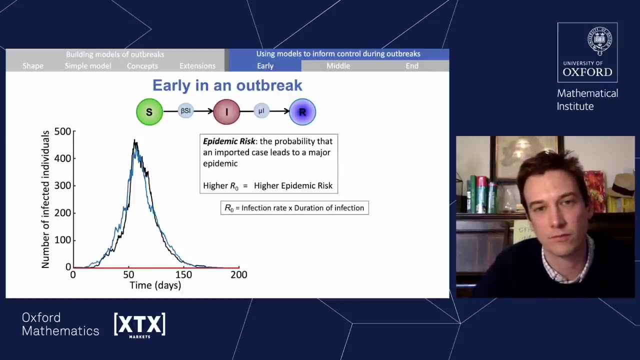 outbreak like the red. Usually the epidemic risk isn't 0 or 1,. instead, the epidemic risk takes a value between 0 and 1, and that value represents the chance that any single imported case will lead on to a large outbreak. The epidemic risk is the probability that an imported case leads on to a major. 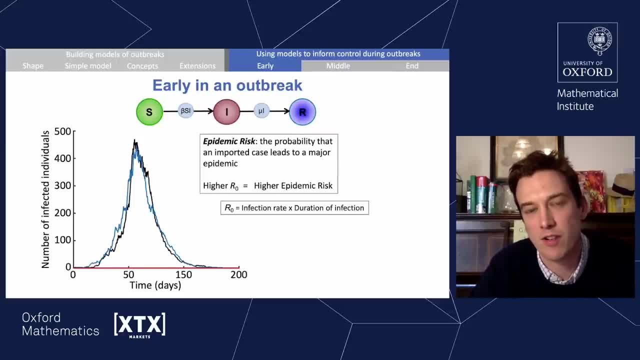 epidemic and if you have a higher value of the basic reproduction number, like we saw before, that means that the disease is more transmissible. if you have a higher value of the basic reproduction number, then you have a higher epidemic risk. in other words, it's more likely that you're going to go on and see an. 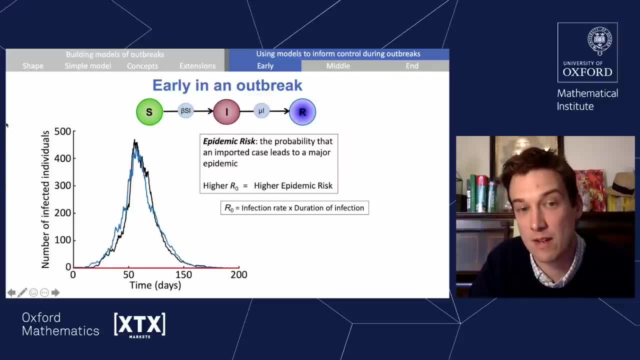 outbreak that looks like the blue or the black, as opposed to the other, to an outbreak that simply fades out like the red. And remember that R0,. so the basic reproduction number could be calculated by taking the infection rate and multiplying it by the duration of. 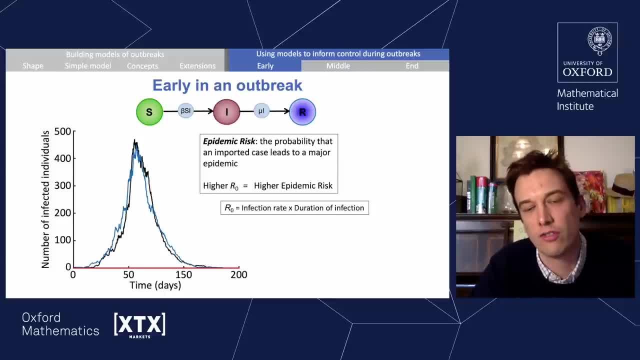 infection. So if you can reduce R0, then you can reduce the epidemic risk. And so, right back at the beginning of the COVID-19 outbreak, when there were very few cases in the UK, only cases that were imported from outside, the question was: well, how can we reduce R0 and therefore reduce 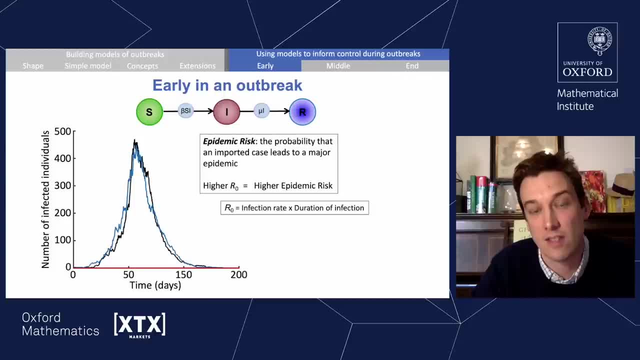 the chance of getting a large outbreak in this country, And the answer to that was: well, either you could reduce the infection rate in some way, or you can reduce the length of time that individuals are infectious for, And so the initial policy in the UK aimed at controlling the COVID-19. 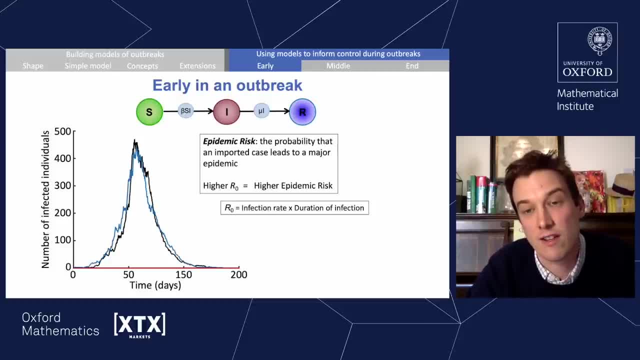 outbreak was to reduce the length of time that individuals are infectious for. So in other words, to go out there and find imported cases and find all of their contacts and make sure that those individuals were isolated quickly. And by isolating those individuals quickly you're reducing the duration of infection for those individuals. You're. 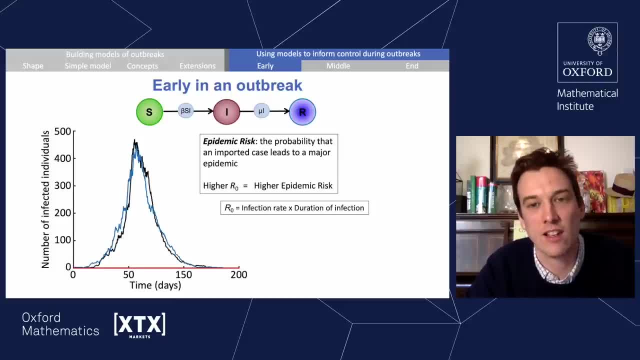 therefore reducing R0 and in turn you're reducing the chance of a large epidemic in the UK. So that was the initial policy. This is a paper that I wrote on this topic right back in January, And the key conclusion is fast. isolation of imported cases can reduce the epidemic risk in countries other than China. So what you need to do is you really need to rapidly isolate any imported case and their contacts if you want to reduce the chance of having a large outbreak in other countries. Unfortunately, what then went on to happen is we did see large outbreaks elsewhere. 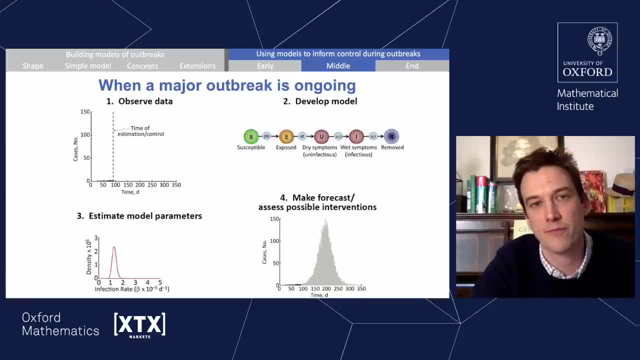 The epidemic risk wasn't reduced sufficiently. What then happens is we enter a different phase of the outbreak. So then the question for modelers is: well, what can we do when a major outbreak is ongoing? And so this is the kind of procedure that we go through. So what we do is we observe data. 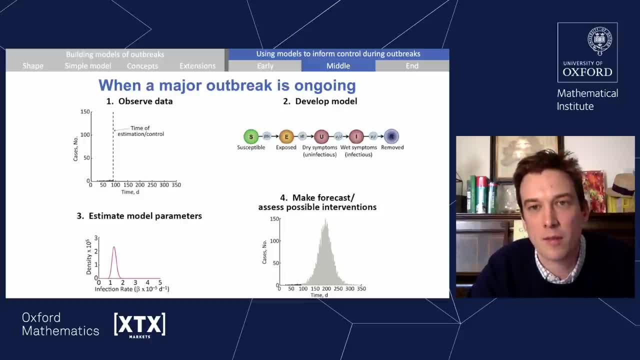 from the ongoing outbreak. We then develop an epidemiological model, so a sort of compartmental model of the type that I showed you earlier. The model I've shown here in step number two is a model that I developed for Ebola virus disease. What we then do is we analyze the model that the outbreak has been in, And what we then do is we 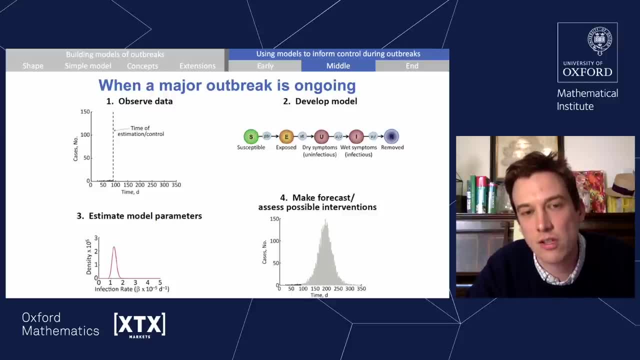 is, we estimate the parameters of the model. so we estimate the values of parameters like the infection rate that we looked at earlier, or like the recovery rate. so we choose those parameters so that the output of the model is consistent with the data that we've observed. and then, once we've got our 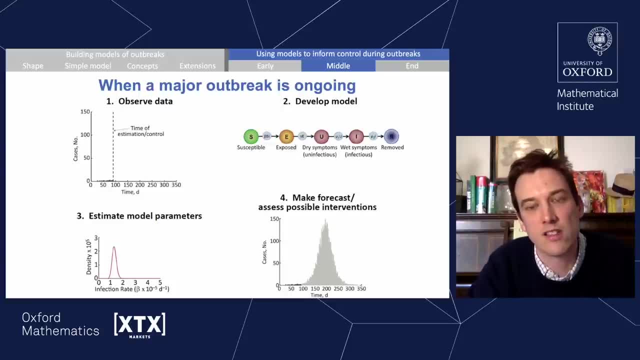 mathematical model. we can run simulations of it forwards to make a forecast and then we can take those simulations and introduce different control interventions in the model and look at what happens in the model under different possible control interventions. and the aim there isn't to predict precisely how many cases there are going to be. 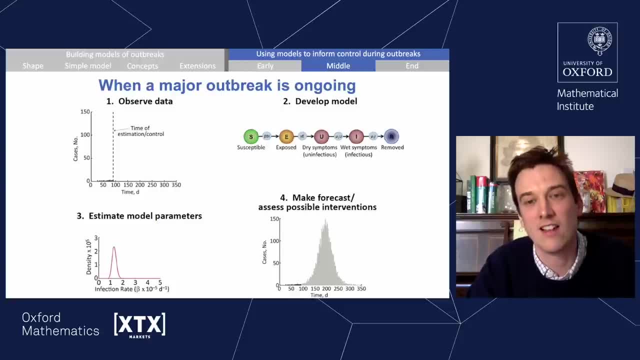 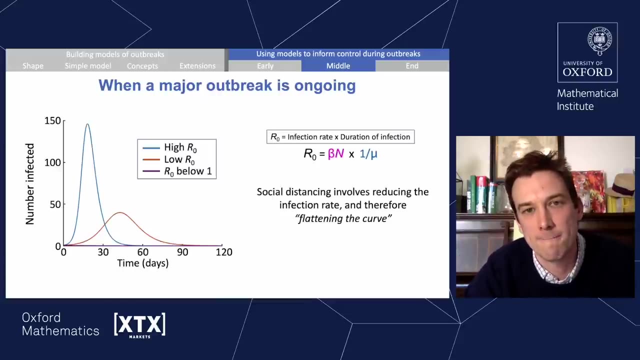 or precisely when the outbreak is going to peak. instead, the aim is to look at different possible control interventions and look at which are most likely to have beneficial effects and which are most likely to have the largest beneficial effects in terms of reducing case numbers, and so these are the kinds of things that one might find. so, again, this is not. 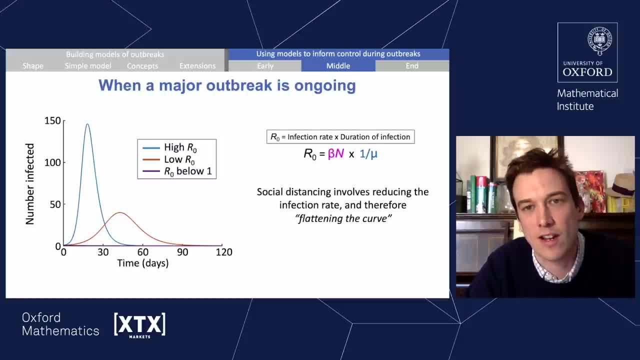 for covid19. this is just general infectious disease outbreak model. something that you might have heard- policy makers, the prime minister's, talked about this a lot- is the idea of flattening the curve. one of the things that we want to do is we want to flatten the curve. 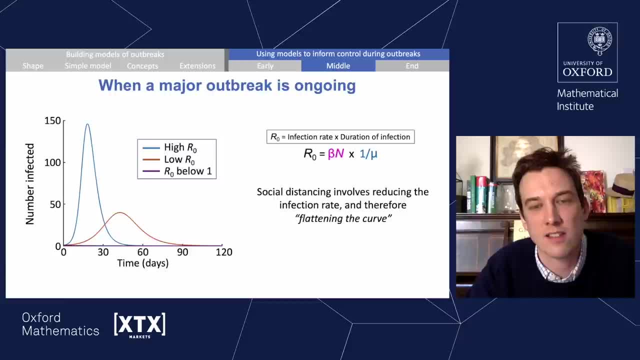 what does that actually mean? well, we can think about that in terms of social distancing. so social distancing involves reducing the rates that we contact other individuals. if we reduce the rate at which we contact individuals, we reduce the overall infection rate because everyone's having a lot fewer contacts. 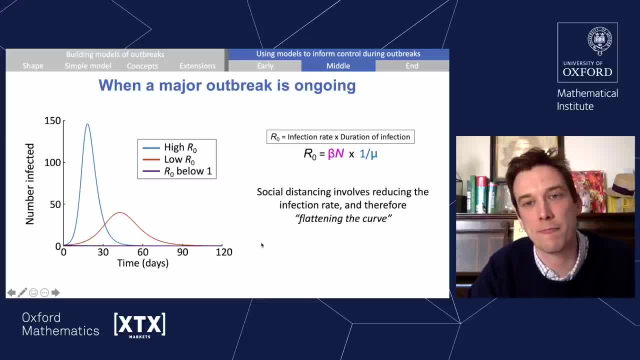 and so we're likely to pass the disease on to fewer people. and so if we reduce the infection rate, what we do is we reduce this parameter beta. and if we reduce this parameter beta, the knock-on effect of that is to reduce r0, because r0 depends on. 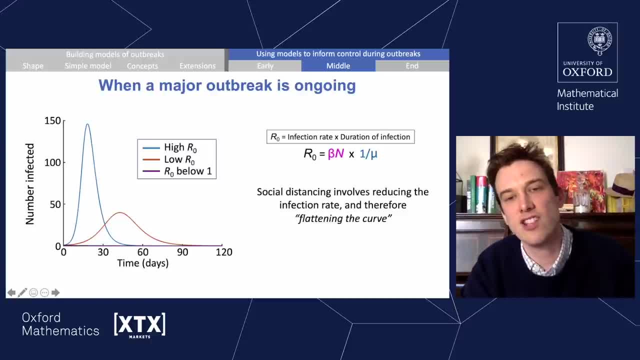 this parameter, beta, and if we reduce r0, what epidemiological models tell us is that we can go from something like the blue curve in this graph to something that's a bit more like the red curve, and this is highly desirable during an infectious disease outbreak, and the reason for that is that 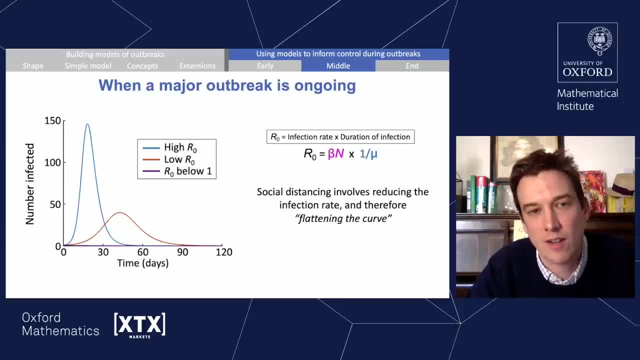 well, one of the key things that you might want to do during an infectious disease outbreak is make sure that the number of infected individuals, at any single time, remains below the capacity for treatment. so, in other words, try and manage the number of infected individuals in such a way that health 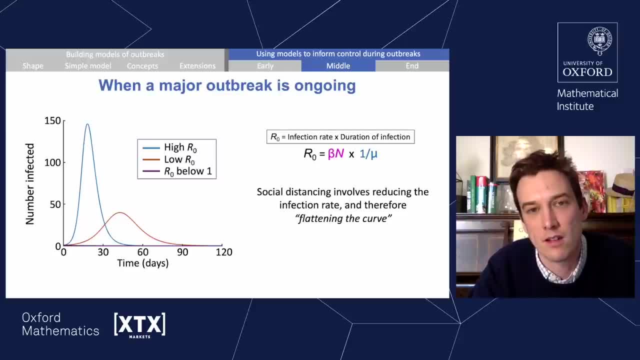 healthcare services can cope. so what you can see here is that in the blue case, so when r0 is high, so without something like a social distancing intervention, the disease sweeps through the population very fast. the peak of this outbreak is very high. what that means is that there's a large 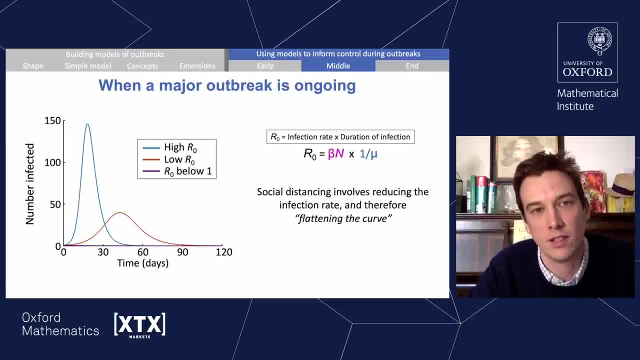 number of individuals infected at any one time and because of that, it's very difficult for healthcare services to cope, because they have to deal with a huge amount of cases all at a single time. in contrast, if you introduce an intervention that reduces r0, that has two effects. firstly, it reduces 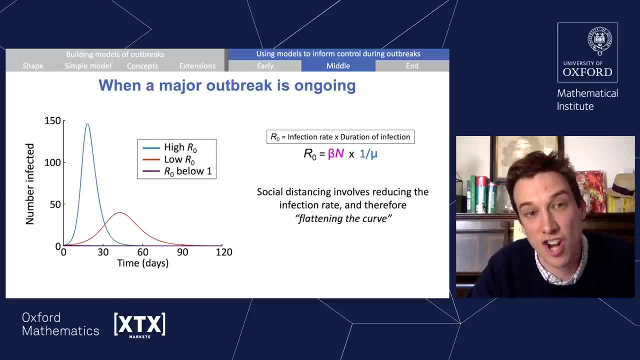 the size of the peak. so if you look at the red curve, then the peak is much lower than for the blue curve. what that means is that at any one time, healthcare services aren't having to treat as many infected individuals, and that's clearly a beneficial thing. but the other thing, the other benefits, 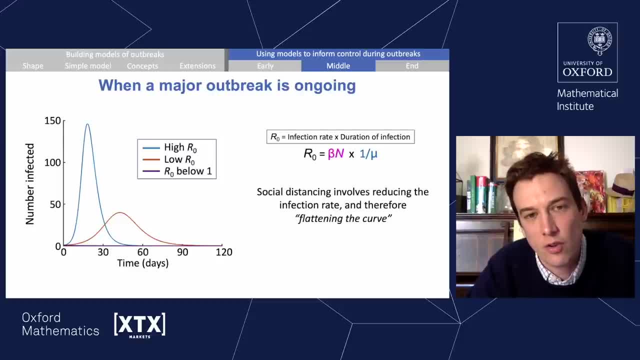 in terms of healthcare services is that if you can reduce r0, then the peak also becomes later, and that's really important because it allows healthcare services more time to prepare for the peak number of infections, and that's a very good thing because it allows healthcare services to increase their 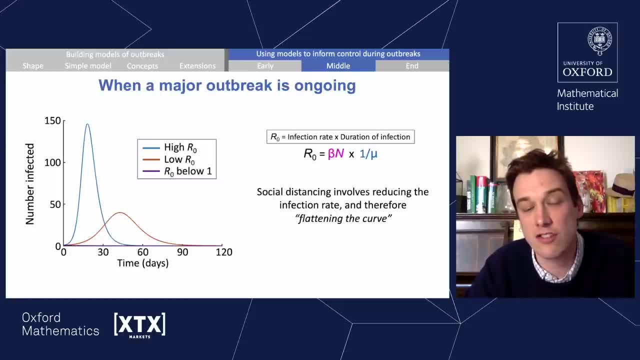 hospital bed capacity. for example, it allows them to distribute personal protective equipment to healthcare workers. it allows them to make sure that they have ventilators, to increase the number of ventilators they have. in other words, it allows healthcare services to better be able to deal with the number of individuals that they 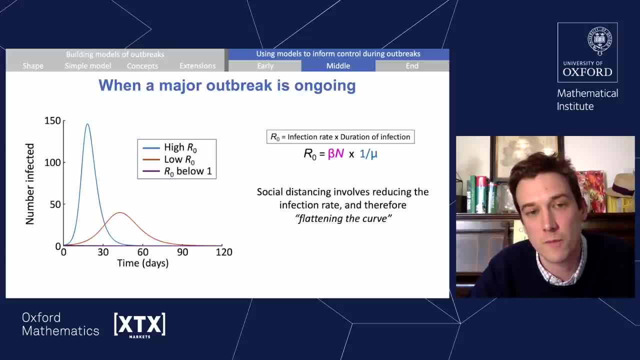 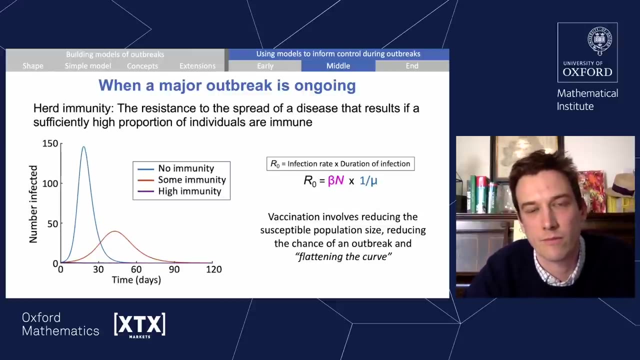 might have to treat so clearly. this idea of flattening the curve is reducing r0, making sure that the peak number of individuals that are simultaneously infected occurs later and that that peak is lower, and that's clearly good for healthcare services. something else we talked about a little bit earlier on is the idea of herd. 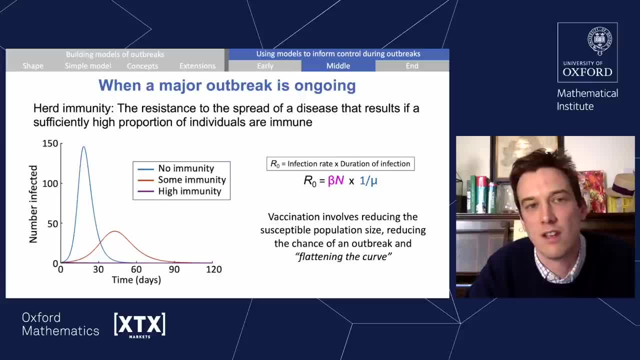 immunity, so the resistance to the spread of disease that results if a sufficiently high proportion of individuals are immune. well, vaccinations: if you've got a vaccination, this actually allows you to increase the number of immune individuals. so remember that we talked about that earlier in the context of r0, so r0 was given by this formula here, where 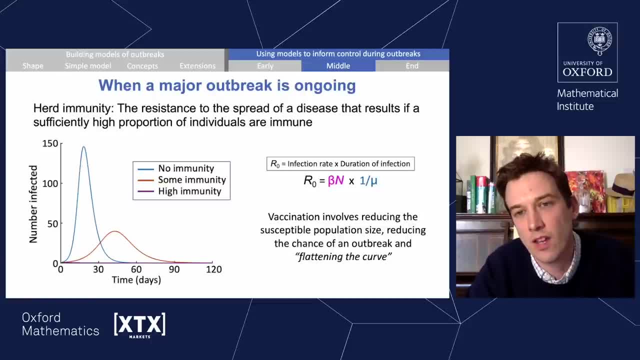 n is the number of individuals that are susceptible to the disease, and if you go and vaccinate lots of individuals, well that reduces the value of n. it reduces the number of individuals that are susceptible to the disease and in turn that reduces r0. and if you reduce r0 again, 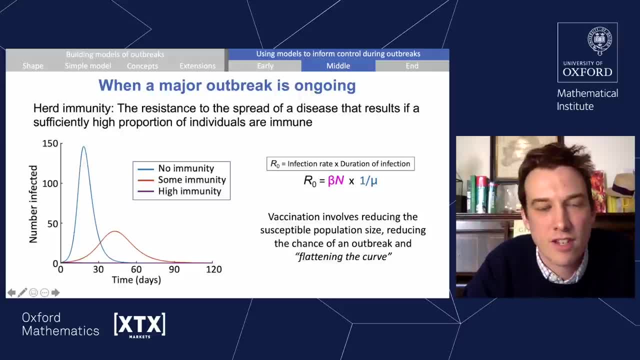 that changes the shape of the outbreak curve, as in this figure on the left. you can go from something that looks like the blue to something that looks a little bit more like the red, and if you can continue to decrease r0, well then the immunity in the population. 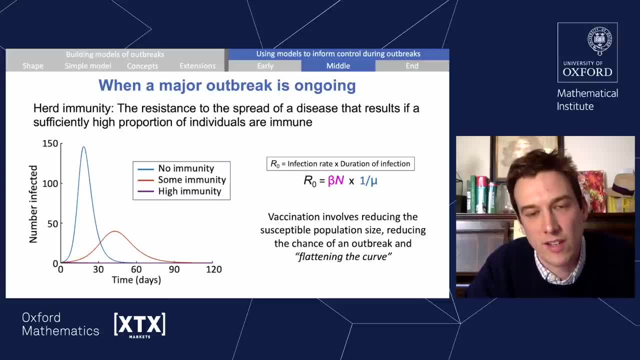 becomes even higher and eventually you get to a point where r0 falls below one and outbreaks can't happen at all. so, hopefully so. i think a vaccine is of the order of a year away. but if a vaccine can be deployed widely in the population for COVID-19, that can prevent this disease recurring in the future. 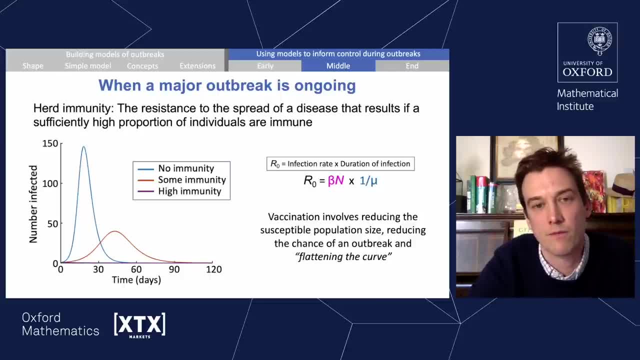 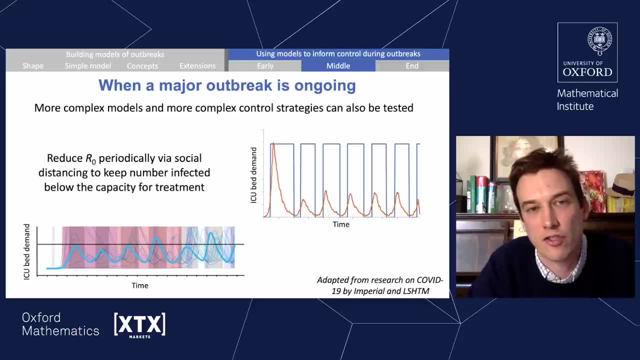 and that's clearly something that's very important. so these two concepts i've just been talking about were in the context of very basic epidemiological models. of course, as i showed you earlier, you can extend these models to become much more complex and with these more complex models, you 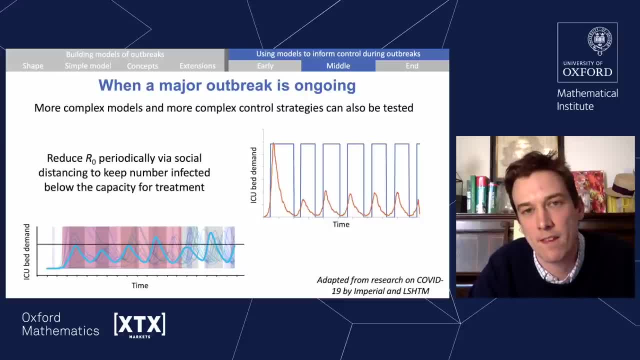 can also test very complex control strategies. so here are a couple of examples for COVID-19. these are the examples of outputs from models that have been developed by Imperial College London, for the graph on the right, and the London School of Hygiene and Tropical Medicine, for the graph. 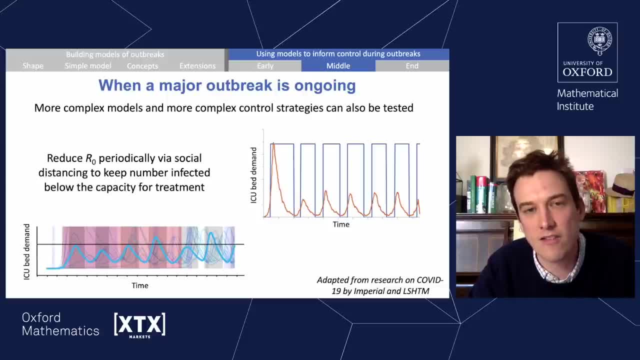 in the bottom left and the idea of these graphs is to test a more complex control strategy. i should say that the London School of Hygiene and Tropical Medicine model in the bottom left. it includes all five extensions to the basic SIR model that i told you about earlier. 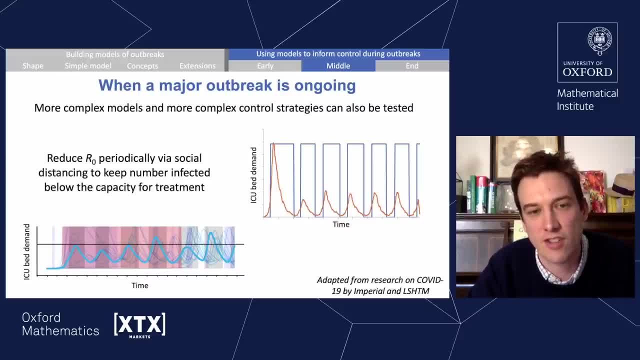 so it's a much more complex model and what you can see here is a quite complex dynamics. so the idea here, so the thing that's being tested, is the idea of reducing R0 periodically by having lockdowns. so having a lockdown for a period of time to reduce the reproduction number. 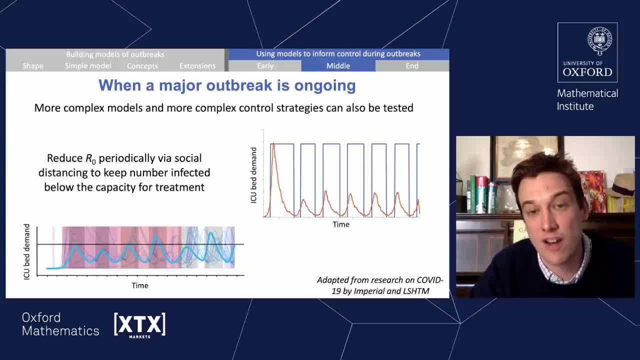 that then reduces the numbers of cases and therefore reduces the pressure on healthcare services. and then you can release the lockdown so that people can go about their daily lives in a more normal fashion. and when you reduce the lockdown, then the numbers of cases goes up again. so, for example, if we look at this graph, 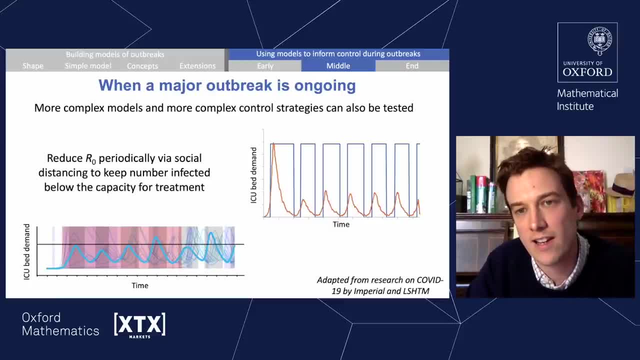 here, so this one from Imperial College London- the blue lines represent whether or not the lockdown is on or off. so in this period here where the blue line is high, then the lockdown is on, and in this period here, the blue line is low and the lockdown is off. 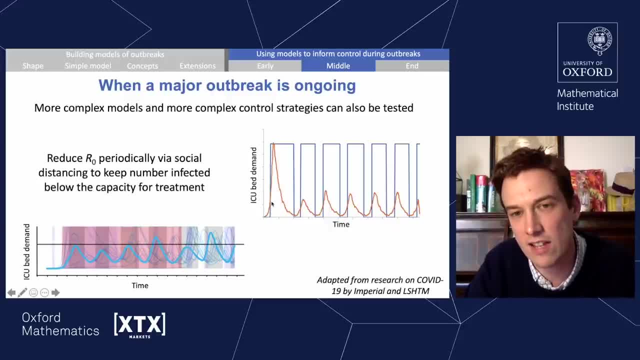 so what you can see in this graph here is that the numbers of cases increases through time. then the lockdown gets implemented, and so then the numbers of cases eventually starts to decline again and it falls back down again to low levels. but when the numbers of cases are, 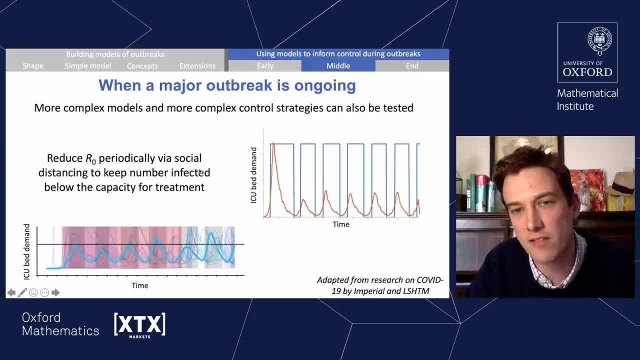 low, then the lockdown can be taken off, but then the numbers of cases increases again. so that's just here, and when the numbers of cases increases again you might put the lockdown back on again to try and manage the numbers of cases you've got and therefore the pressure on healthcare services. 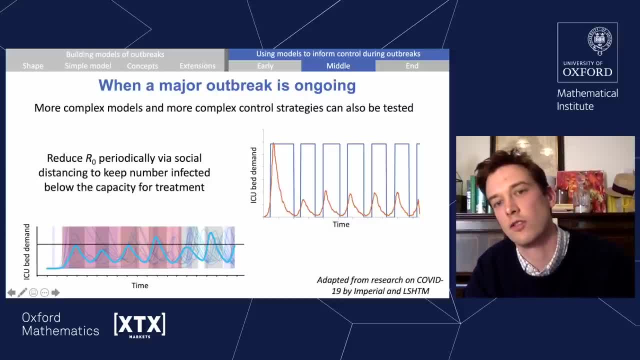 that's when the lockdown's back on again. then the numbers of cases falls back down again, and so on, and you see this repeating pattern where you put the lockdown on, cases fall down again. you take the lockdown off, cases increase. you put the lockdown on again cases. 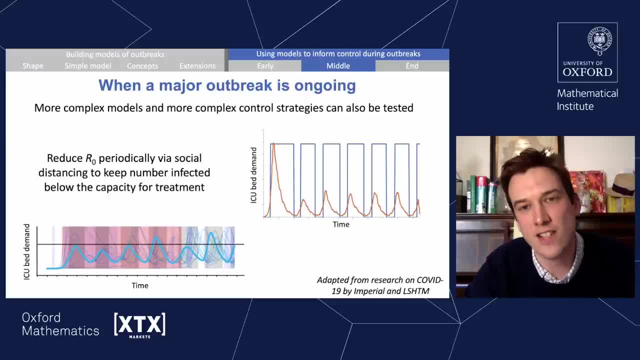 fall down again and so on, and the benefit of this kind of strategy is that it is it allows you to manage the number of cases of disease at any particular time, and by doing that, you can keep the need for intensive care unit beds low enough so you can keep the number of infected individuals low enough. 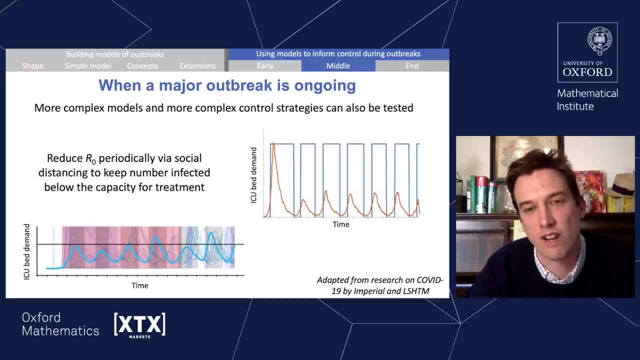 that hospitals are able to cope with the number of individuals requiring intensive care unit beds. so that's kind of more complex model and a more complex control strategy. and you see a similar thing from the london school of hygiene and tropical medicine model in the bottom left. you put the lockdown on. the cases fall down again, you take the lockdown off. so 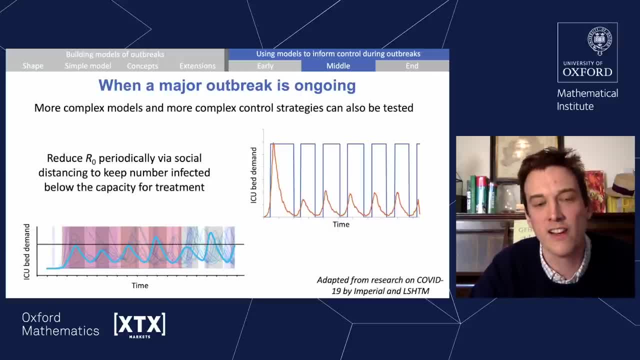 that people can go about their everyday lives in a more normal fashion, and then cases go up again and so on, and you repeat, and you get this kind of oscillatory behavior which in theory might be able to keep the bed demand in intensive care units below the number of intensive care unit beds. 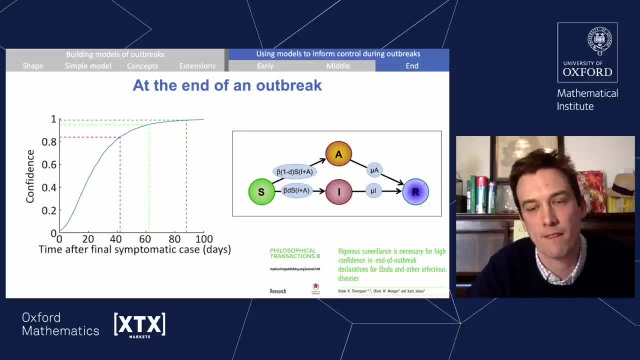 that the healthcare service has okay, so that's something a little bit about how models can be used when outbreaks are ongoing, when you can't see any more cases, so when we're right towards the end of an infectious disease outbreaks, models are still useful. so this is an example of some work that we did. 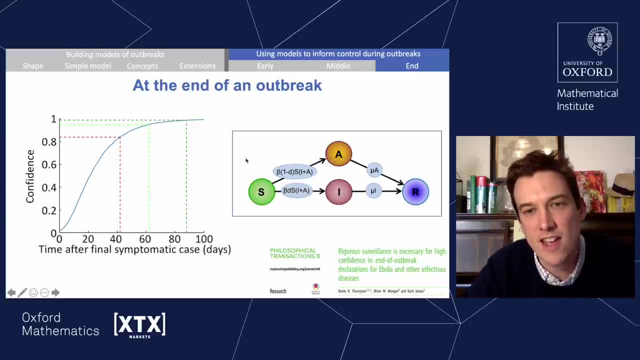 for ebola outbreaks, and the idea here is that we have this model that we've been talking about for a while now, that we have this model which i showed you earlier, this model in which it's an sir model, but there are also individuals that may not be reporting disease. 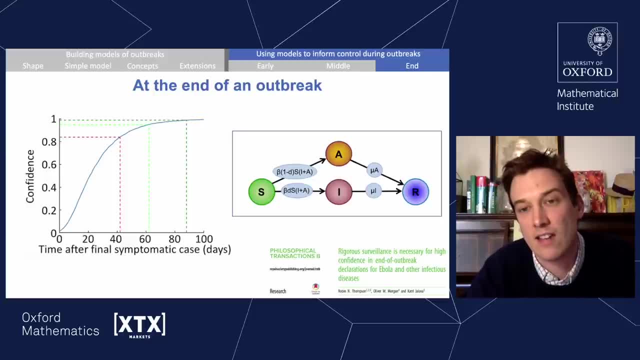 so in other words, you have asymptomatic infections which don't get recorded in routine surveillance data. so in other words, you can be in a situation where you haven't seen any cases for the last five days, but there may still be cases out there because there are these asymptomatic. 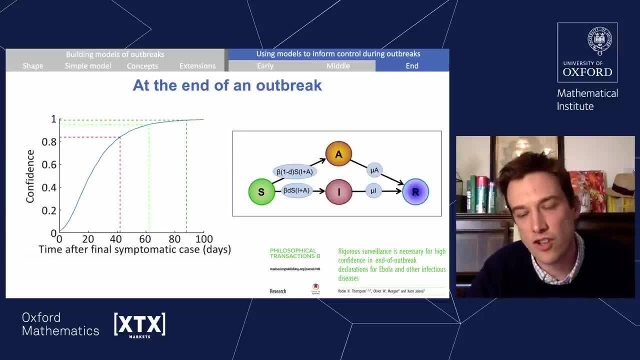 infected individuals that you simply don't see. in fact, i won't go into too much detail about that, about this, but what you can do is you can use mathematical models to say: well, if we haven't seen any cases for the last 10 days, let's say 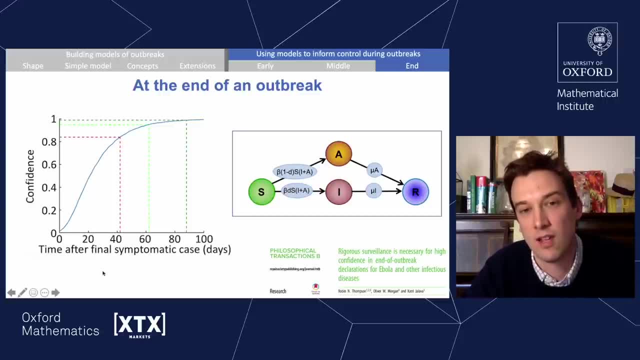 how likely is it that the outbreak really is over? and so we developed this figure for ebola outbreaks, which shows that if you wait a long time without seeing any symptomatic cases, well then you can be very confident that the infectious disease outbreak is over. but if, in contrast, you only wait for a short time, so let's say it's been five. 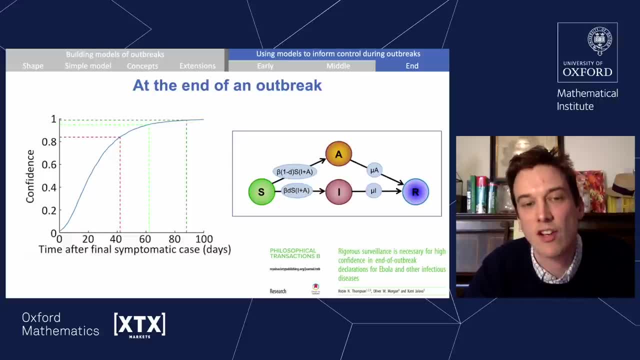 days since you last saw a symptomatic case, well then you can't be very confident that your ebola outbreak is over. if you wait for the sort of who guideline period before declaring an ebola outbreak over, then this very simple outbreak model suggests that. well, after 42 days, which 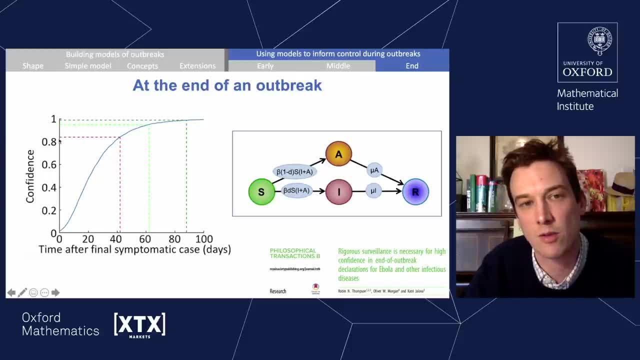 is the who guideline before declaring an ebola outbreak to have finished. there's approximately an 82 percent chance that that ebola outbreak really is over and about an 18 percent that the outbreak in fact isn't over and that there are still hidden cases out. 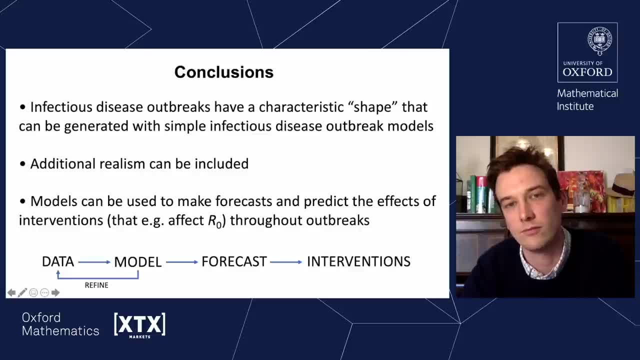 there that you just can't see, okay. so to conclude then: so we've talked about infectious disease outbreak modeling and we've said precisely what an infectious disease outbreak model is. we've shown that infectious disease outbreaks have a characteristic shape. the numbers of cases in a single wave outbreak goes up, it peaks and then it comes back down again. 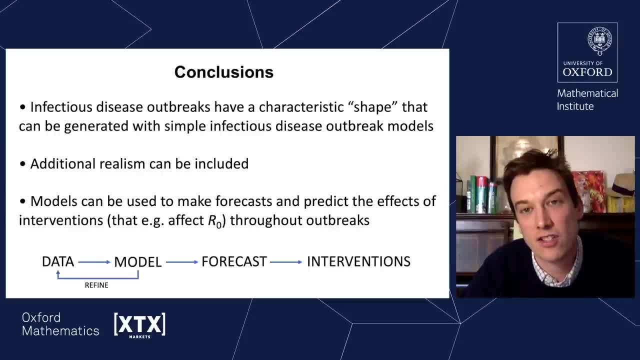 to near zero. even very basic infectious disease outbreak models can capture that kind of characteristic shape. those models can then be extended to include additional realism, so things like, for example, transmission from individuals that aren't showing symptoms, or things like different transmission rates between individuals in different locations. 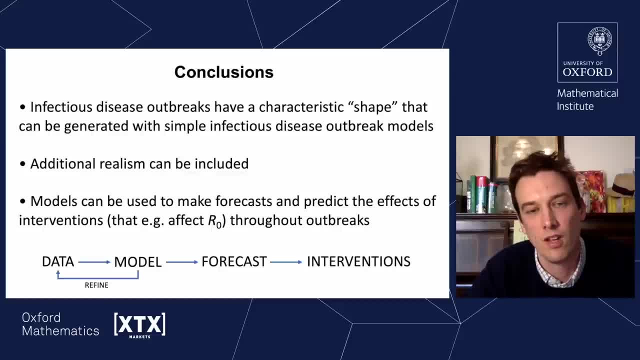 or individuals of different ages. we've then talked about how models can be used at different stages of an outbreak for doing various things, including making forecasts and predicting the effects of different potential control interventions, for example, interventions like social distancing that affect the reproduction number, and the idea behind 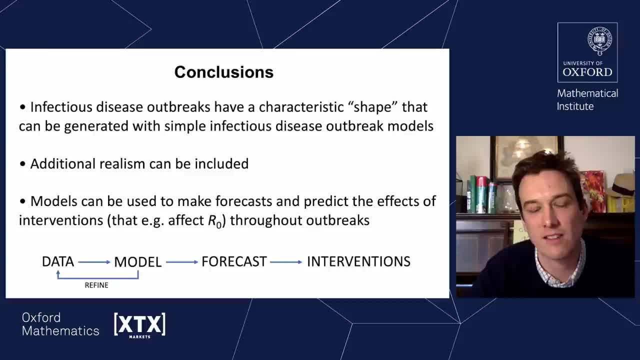 using mathematical models for making forecasts and predicting the effects of different interventions is shown at the bottom. so you have some data from an ongoing outbreak. you then develop a mathematical model that can rep, that can reproduce those data. you refine the model to make sure that the model can reproduce the data more. 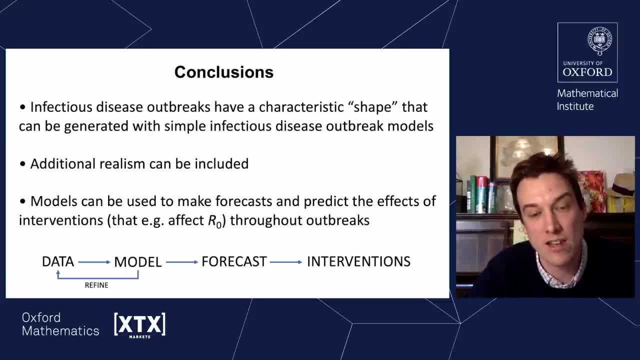 accurately, and you also refine the model as more data come in during the outbreak. once you've got the model, you can then use simulations forward to generate a forecast as to how many cases you might expect to see going forwards, and then you can introduce different public health measures.